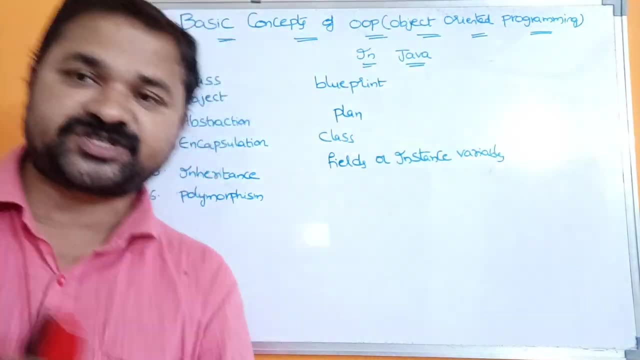 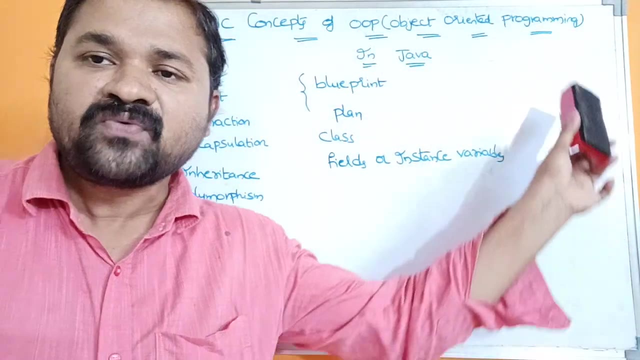 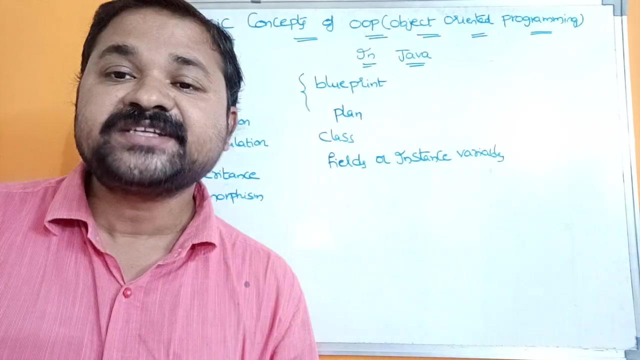 then we can create n number of objects. once we have blueprint, then we can create n number of houses, n number of houses based upon our blueprint or the plan. so these three are the major definitions for a class. the first definition is: a class is a blueprint from which an object is. 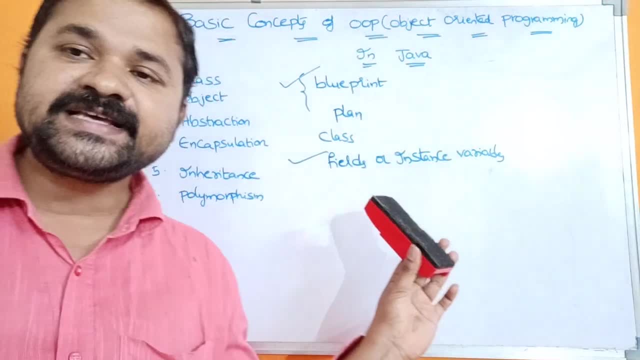 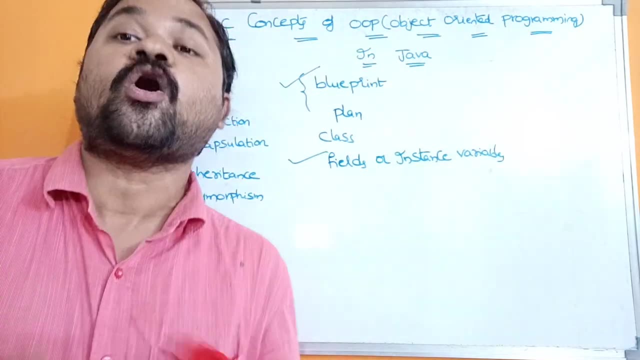 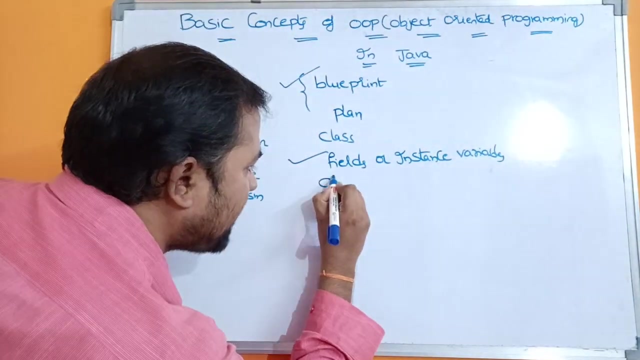 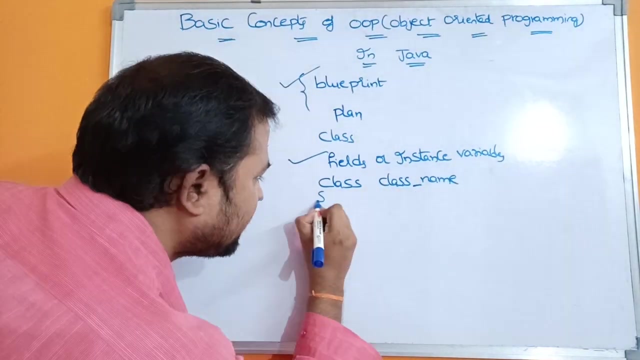 created. the second definition is: class is a collection of fields and methods. the third definition is: class is a collection of objects. now let's see the syntax for declaring a class in java programming language. we can declare class with the help of a keyboard called class, class, space, class name. within the curly braces we can have fields as well as methods. 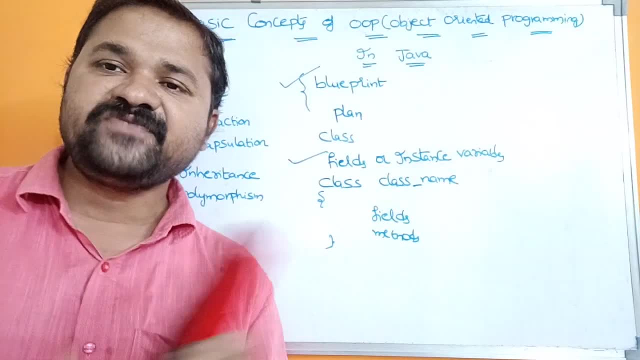 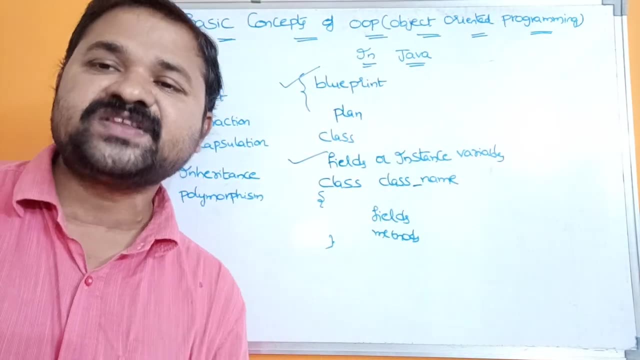 we can have fields as well as methods for class name. we have to follow the naming conventions for the class. we know the naming conventions for a class. the class name always begins with uppercase letter and the first letter of every inner word begins with uppercase letter. so let the class name. 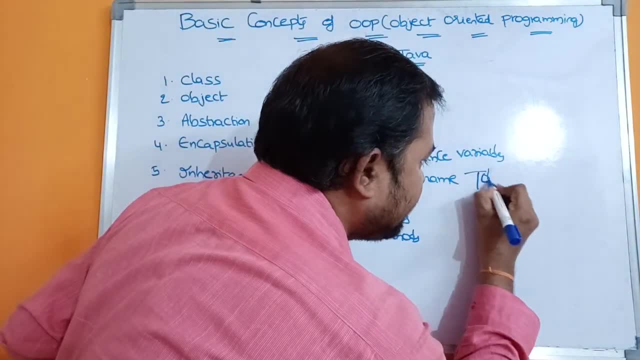 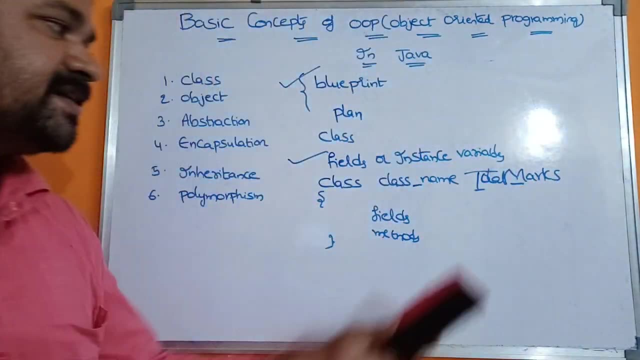 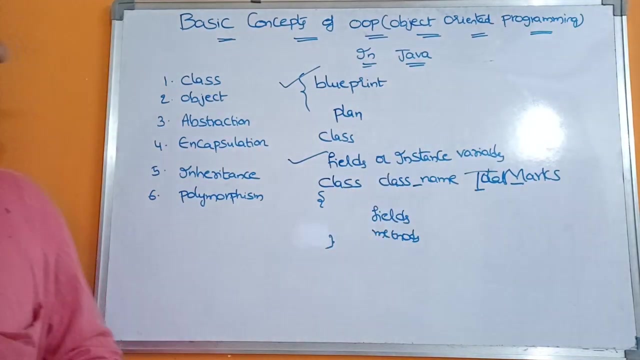 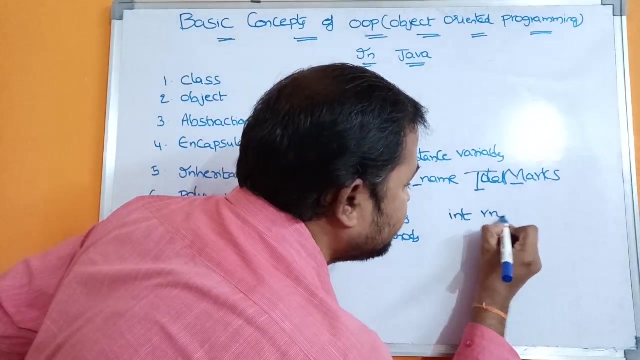 is total marks, then t should be uppercase letter as well, as the first letter of every inner word is uppercase letter. so this t and m are uppercase letters, whereas the remaining letters are lowercase letters. let us assume that here, the here we have fields like rule number, rule number, let the rule number is of type some integer. let we have a field like: 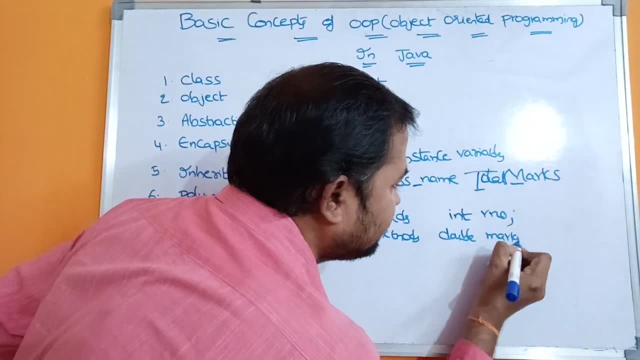 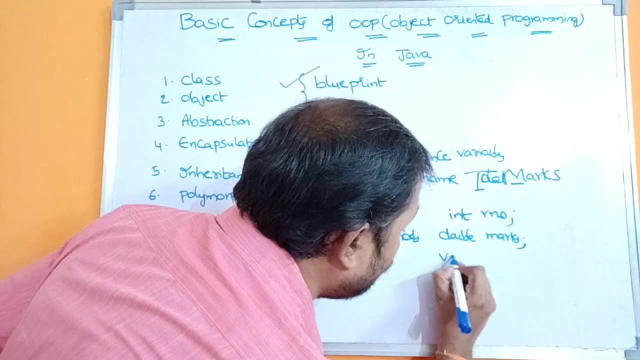 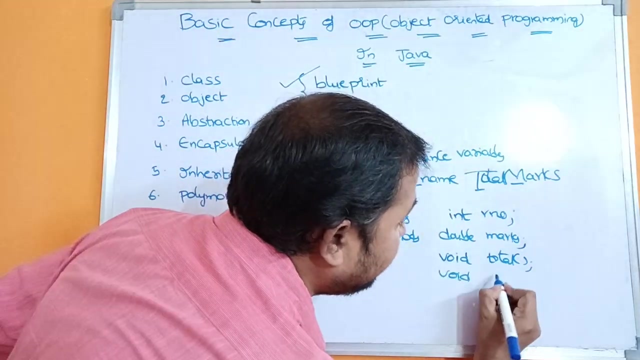 marks, so double marks. so these are nothing but fields. likewise, we can have some methods. okay, let us assume that we want to calculate some total, so void total. next, let us assume that we want to calculate some average, so void a, b, c. so these are nothing but the methods to calculate. 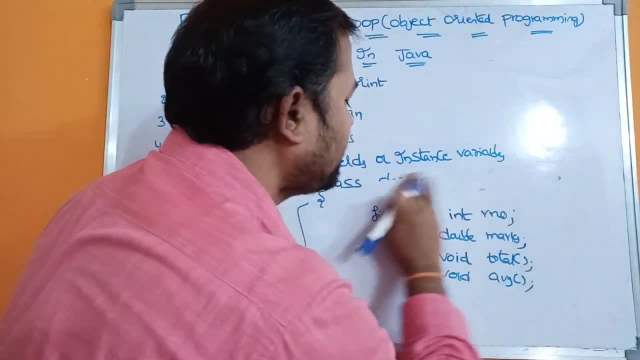 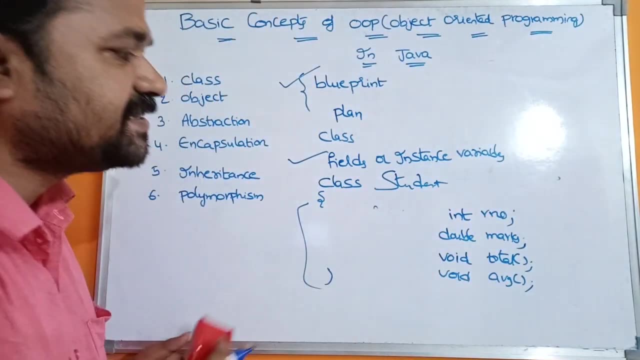 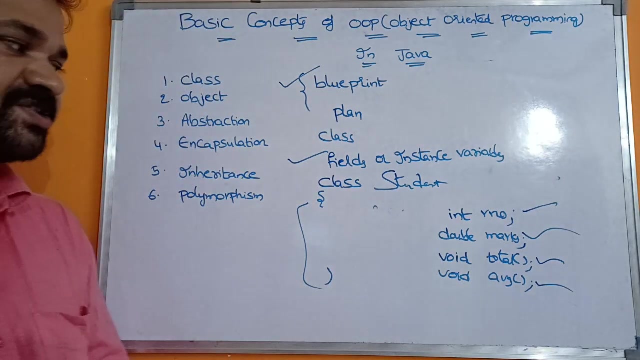 methods. so let here the name of the class is: instead of total marks, it is better to take student student. so what are the fields here? the fields are nothing but rule number and marks are nothing but the fields, whereas total and abc are nothing but the methods. so this class contains: 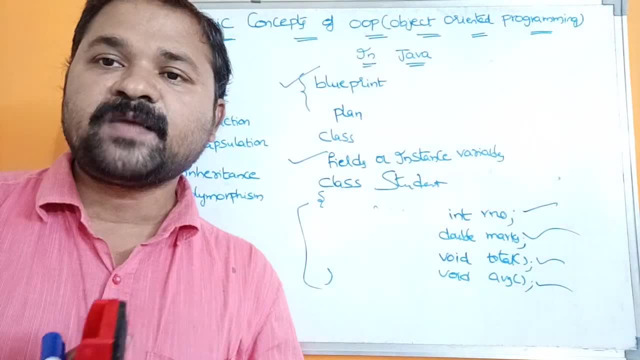 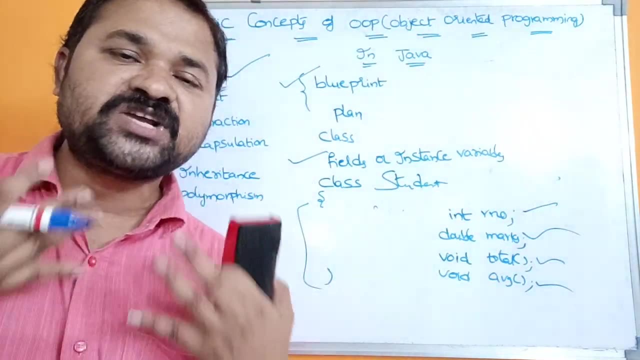 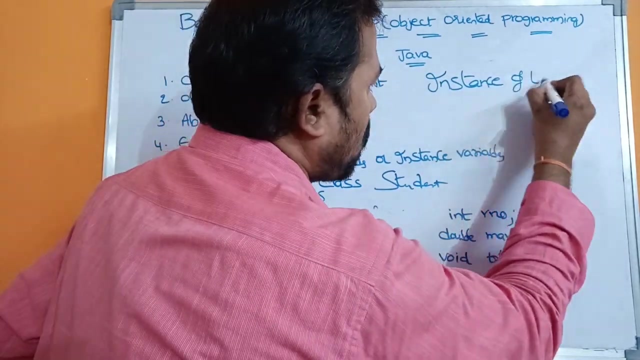 these two variables, as well as these two methods. so this is about what is a class? now let's see the second one. the second one is object. the major, important definition for object is: object is instance of the class. so this is very, very popular definition: object is instance of the class. 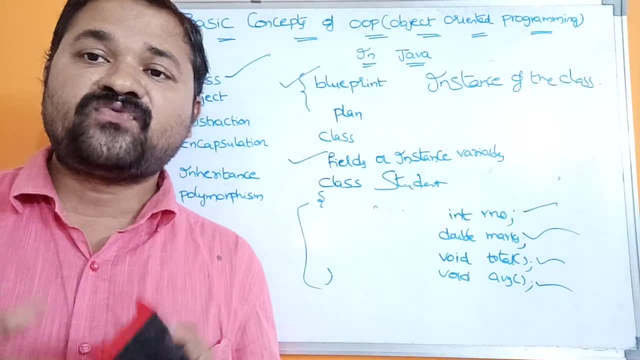 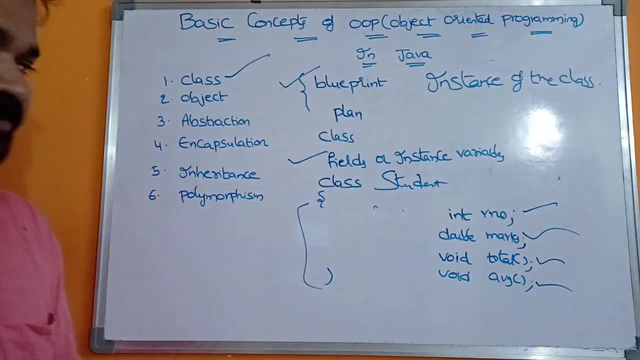 once a class is created, once a class is declared, then memory will not be allocated to the member variables of the class. so once this class is declared, then memory will not be allocated for rule number and marks. so this is the second one. the second one is object: the major important. 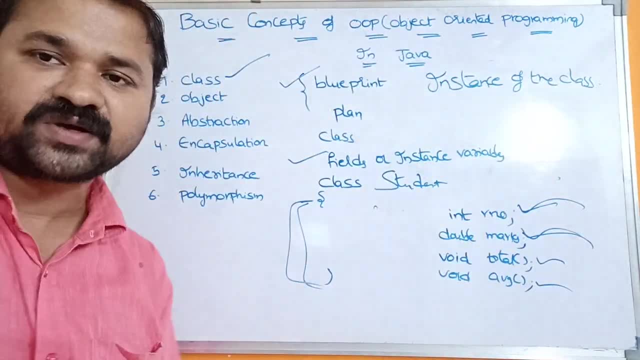 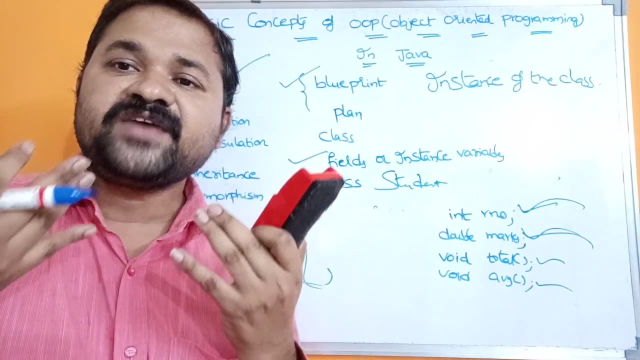 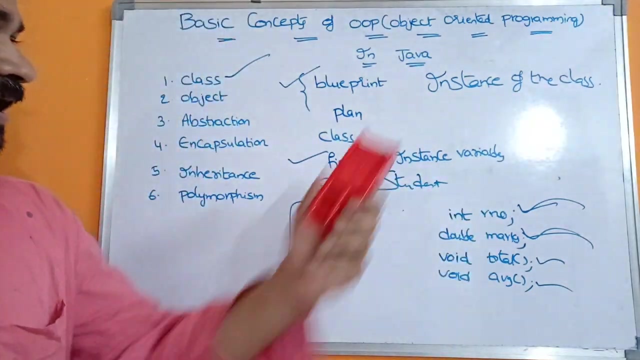 definition for word type as well as the memory will not be allocated for the marks, so the memory will be allocated only when an object is created. so we can say that whenever an object is created, then only memory will be allocated to the variables of the class. okay, let's see the syntax for creating an object. the syntax for creating an object is class name. 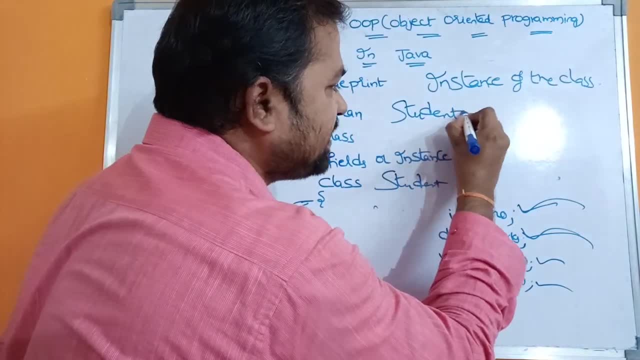 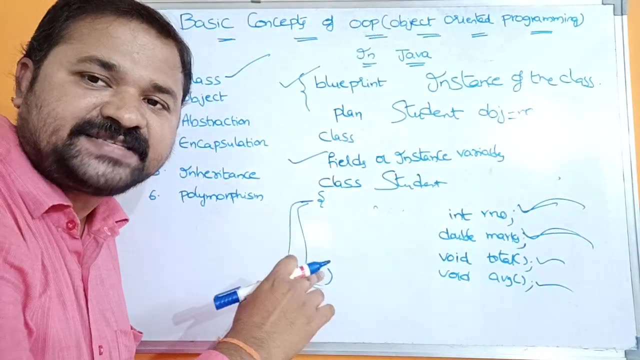 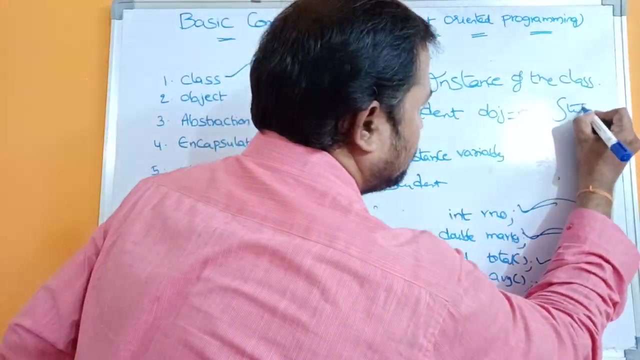 here what is the class name? student is the class name. so class name space object is equal to. here we are using an operator called new operator. so class name space object is equal to new class name. so here, what is the name of the class student? so new student. here we have to use. 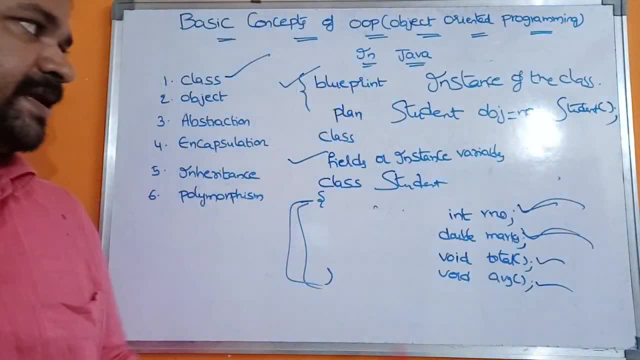 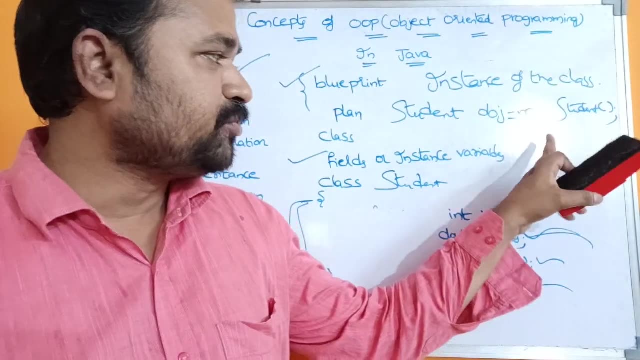 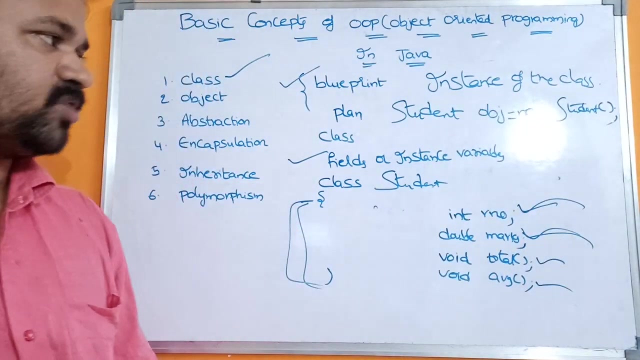 this: left parenthesis, right parenthesis ends with semicolon. so class name is the student space. let name of the object is govijay is equal to, we have to use a keyword called new, next class name. after that we have to use this: left parenthesis, right parenthesis ends with semicolon here: new operator. 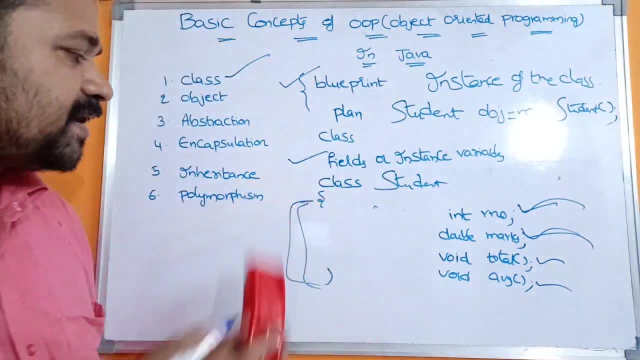 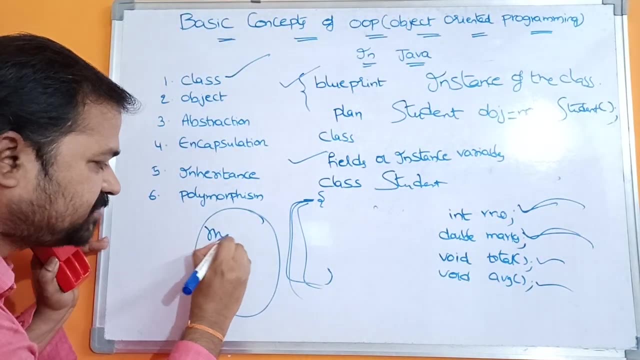 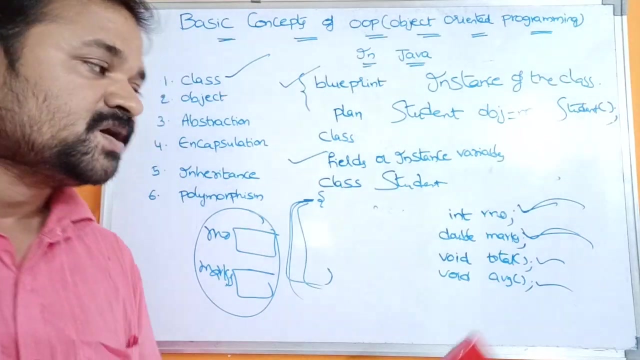 allocates memory for the object. here. what are the variables of the class? we have rule number as well as mocks. so this is nothing but our object. so our object contains rule number as well as mocks. in java programming language, the size of the integer is four bytes, so four bytes of memory. 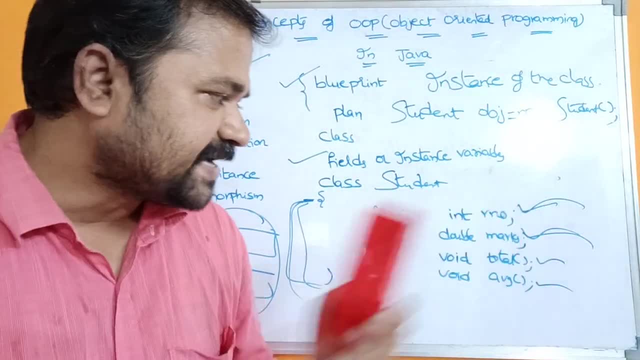 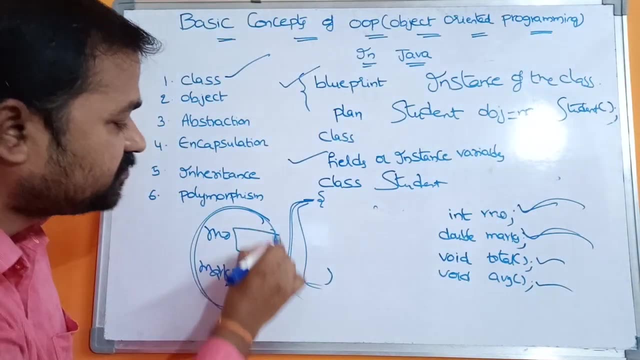 will be allocated for the rule number as well as let. the size of the double is eight bytes, so eight bytes of memory will be allocated for the mocks. okay, so this is nothing but our object. so our object contains these two member variables. so, with the help of our object here, what is the? 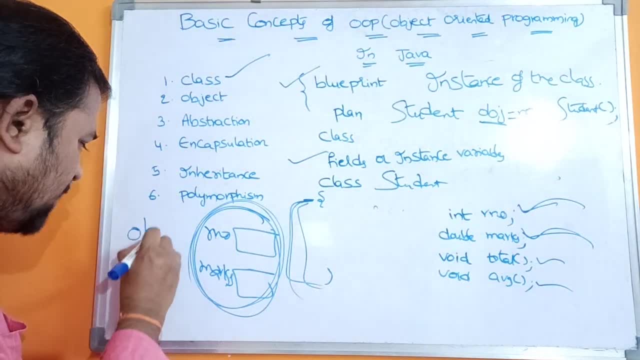 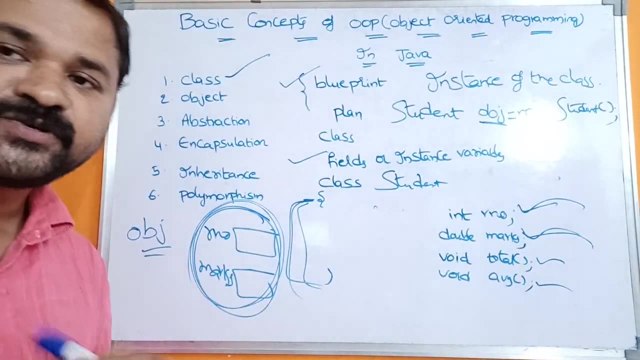 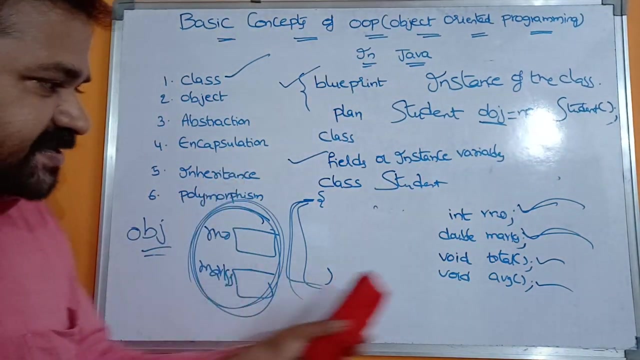 name of the object. govijay is the name of the object. so with the help of the object we can access variables of the class as well as methods. okay, so object mainly contains variables as well as methods, so by using object we can access these variables as well as. 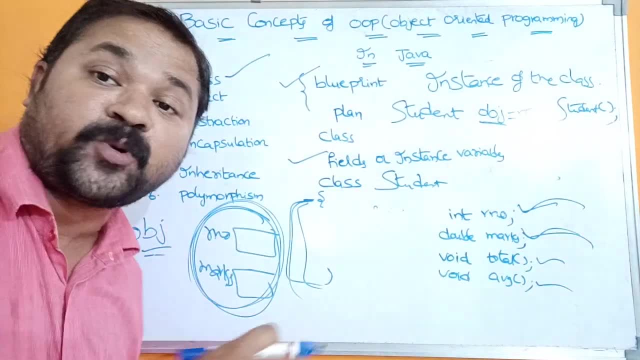 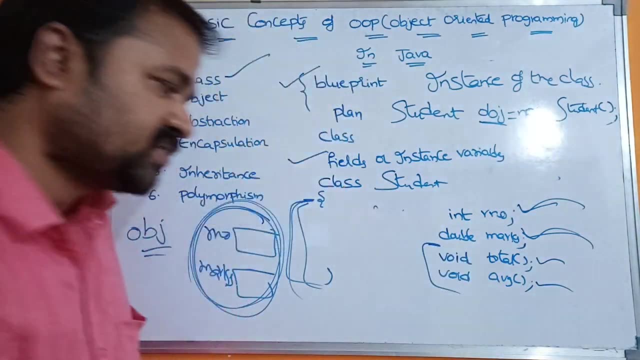 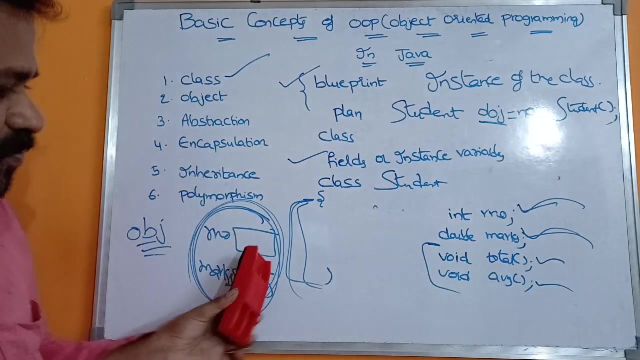 methods. these variables can also be called here as properties. properties are nothing but the variables of the class, whereas these are nothing but operations. so in order to perform the operations we use the methods. so by using object we can access the variables as well as we can access 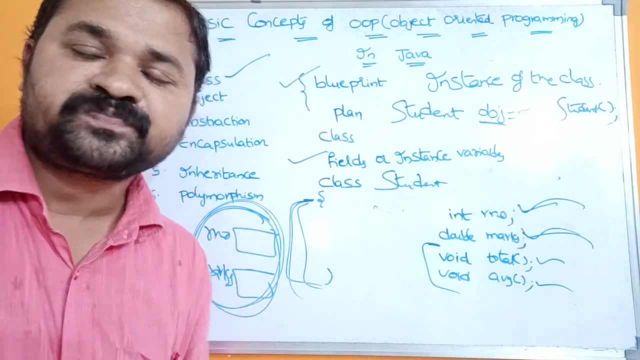 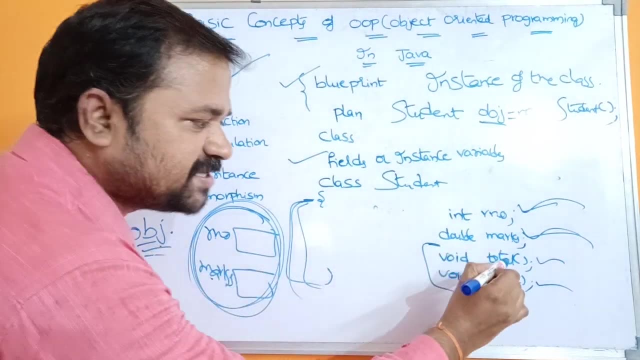 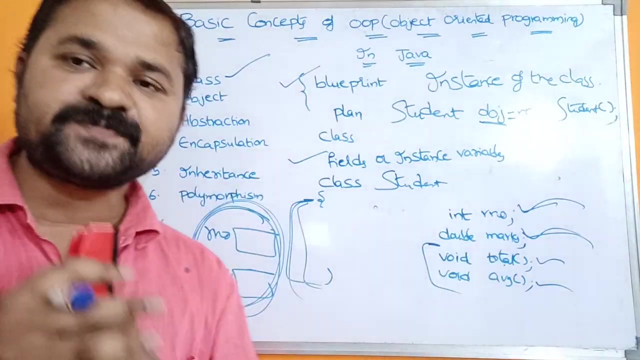 the method. here we use dot operator in order to access the variables as well as methods. so obz, dot, rule number mobocrt, objmox, objtotal objabj. like that we can access variables as well as methods. So already we have seen one definition for the object. 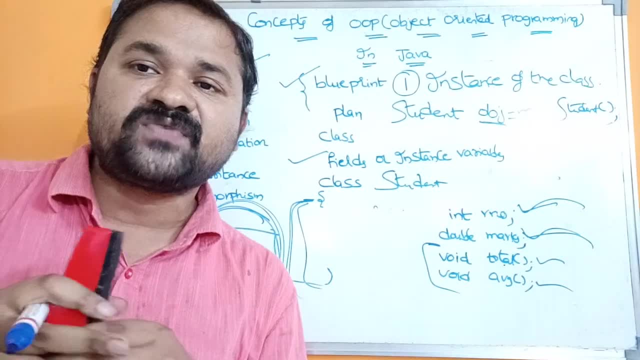 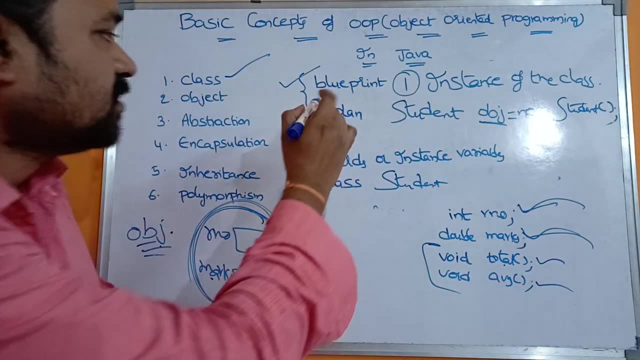 So what is the first definition? Object is instance of the class. Let's see the second definition, object. Already we have seen one example. So once a class here. what is a class? A class is a blueprint from which an object is created. 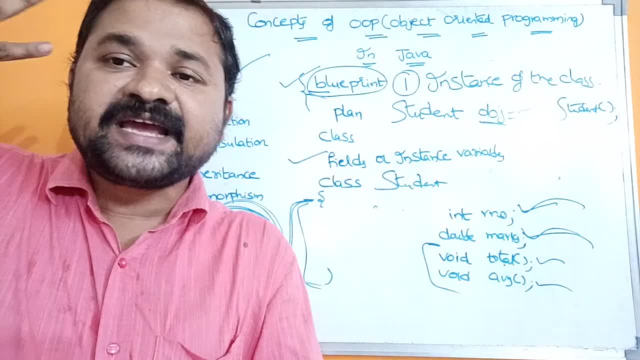 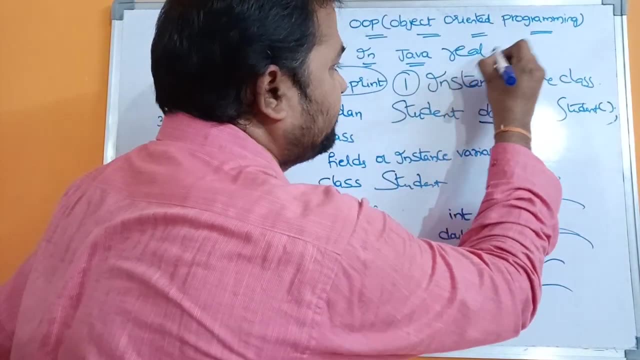 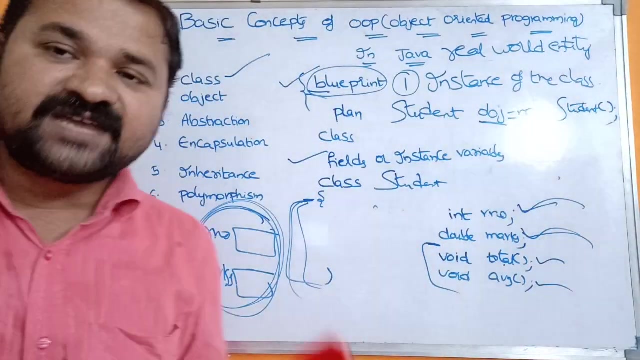 So if we take the example of a house, So that constructed house is nothing but object. So object is real world entity. So this is the second definition: Object is any real world entity. So that means any entity. anything that we will see in the world is nothing but an object. 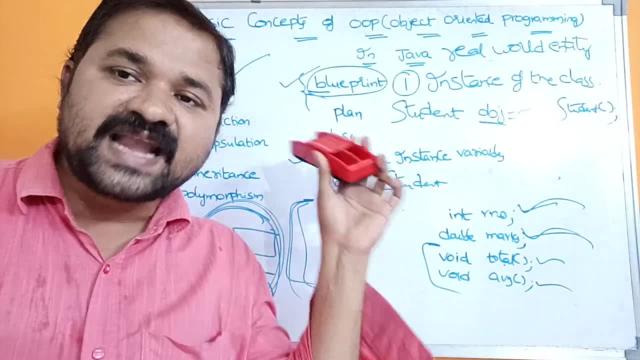 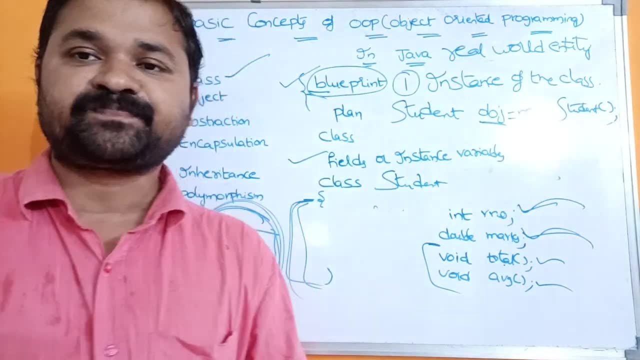 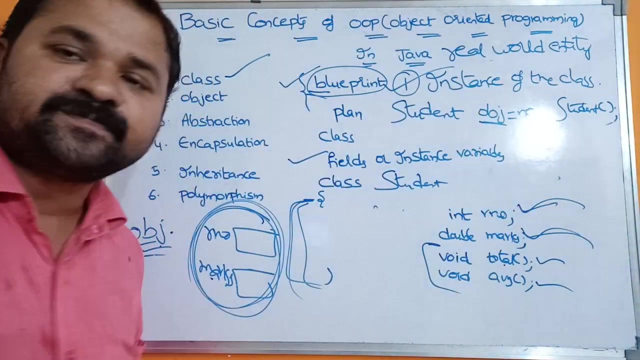 Object is a physical entity Where he has class is logical entity. Physical entity means the entity that has physical existence. So here there are three important definitions for the object. The first definition is: object is instance of the class. The second definition is: object is any real world entity. 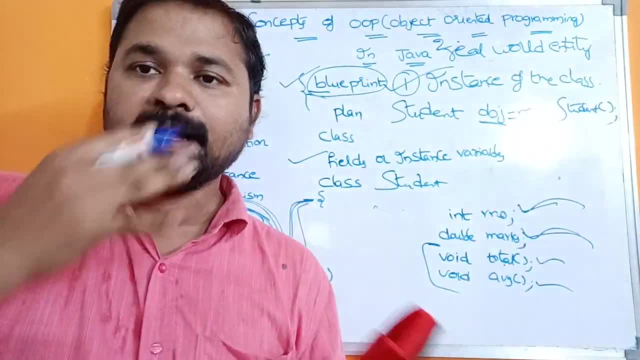 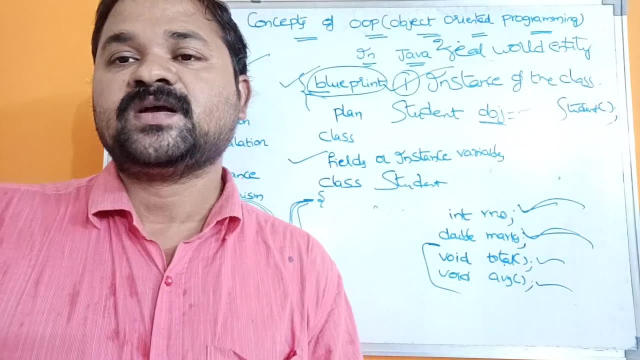 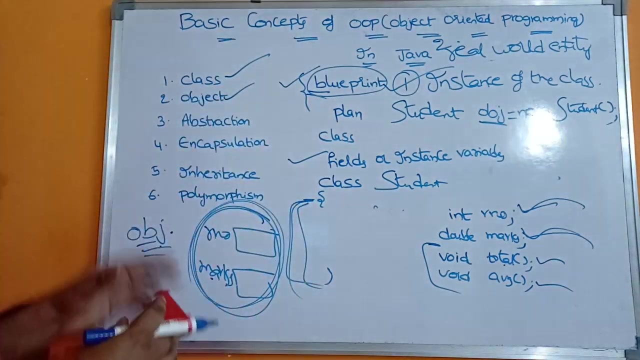 Any entity that we will see in the world is nothing but an object, And one more important definition is: object is physical entity. Where he has class is logical entity. So this is about what is a class and what is an object. Now let's see the next one. 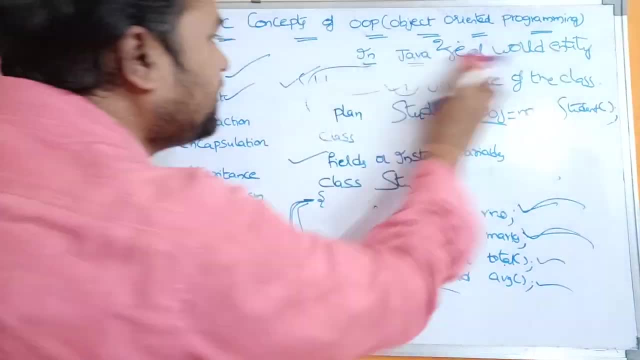 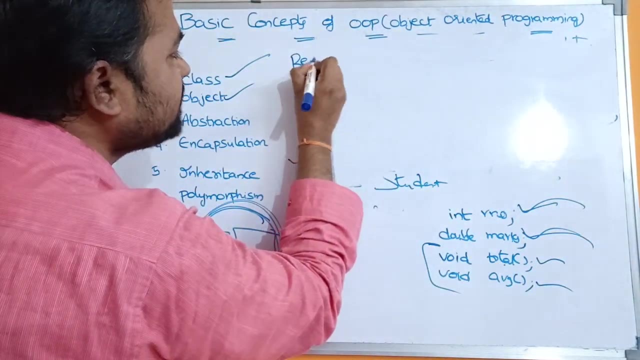 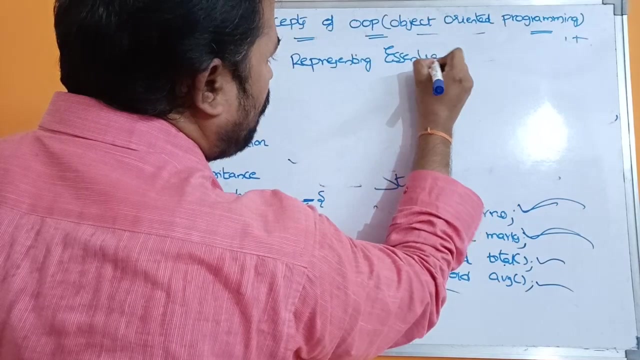 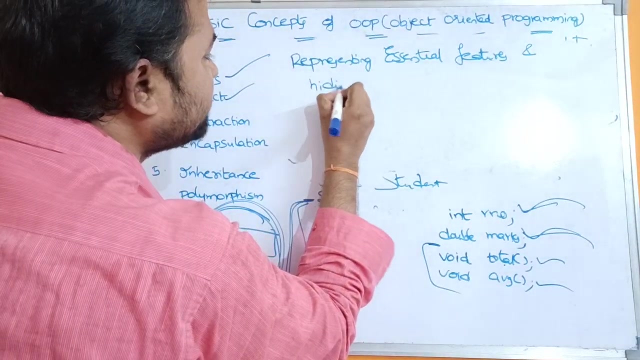 So the next one is abstraction. So let's see the definition for what is an abstraction. Abstraction means representing essential features. Representing abstraction is the concept of representation, Representing essential features and hiding implementation details and hiding implementation details. So this is the definition for abstraction. 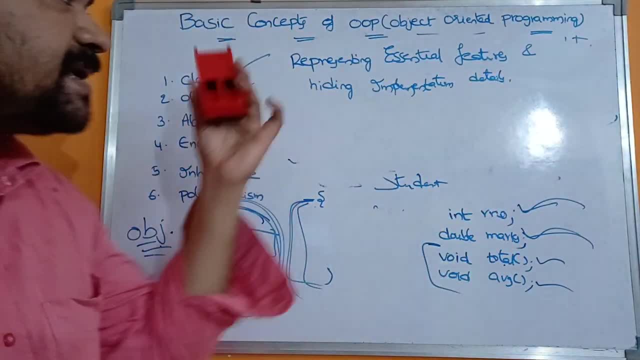 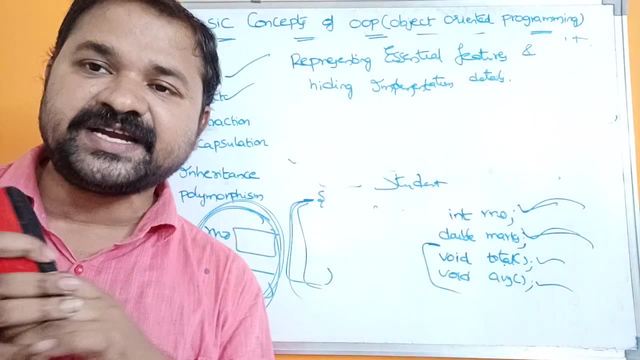 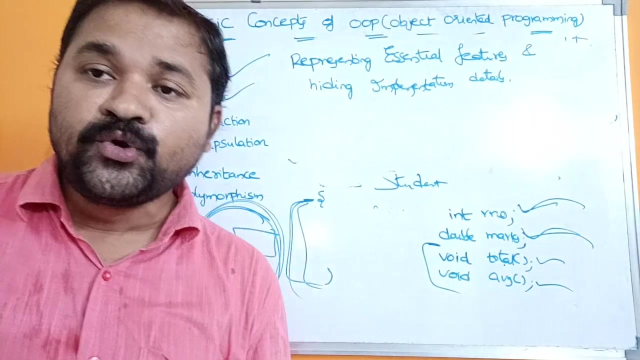 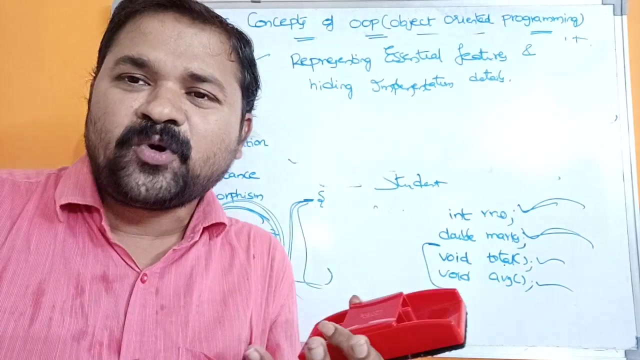 So abstraction is the concept of representing essential features and hiding the background details. That is nothing but hiding implementation details. If we take the example of a bike, we can drive the bike, But we don't know how the components like clutch, gates, brakes, so all those components work. 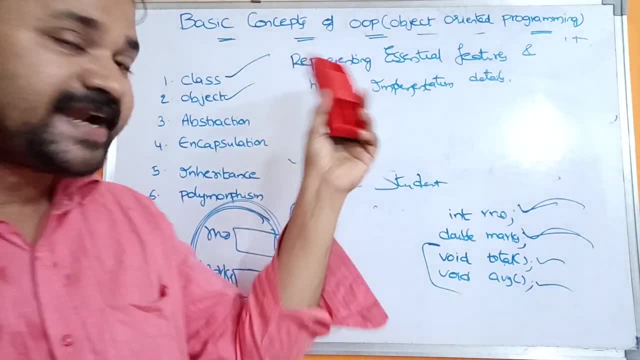 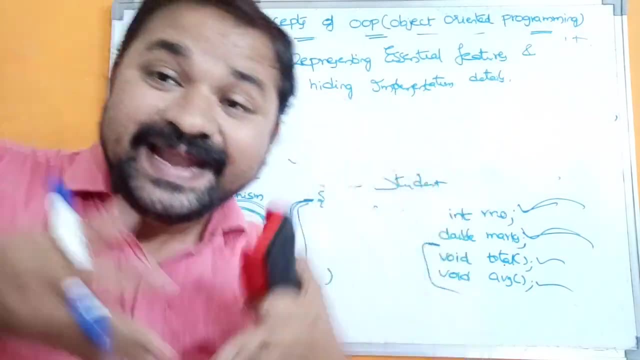 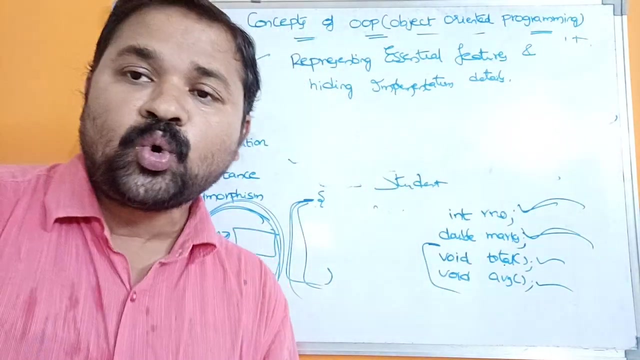 We don't know all those details, So that is nothing but abstraction. Here we can drive the bike, but we don't know how all those components are internally implemented. We don't know how the brakes are implemented. We don't know how the clutch is implemented. 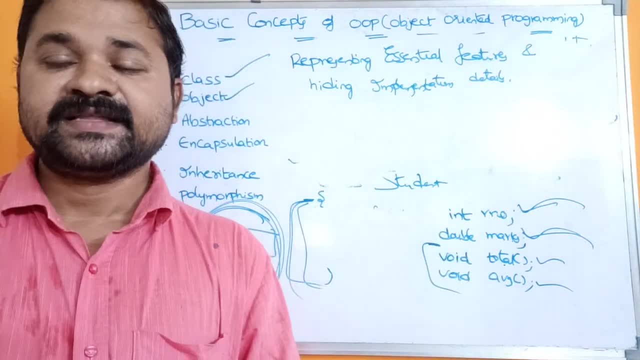 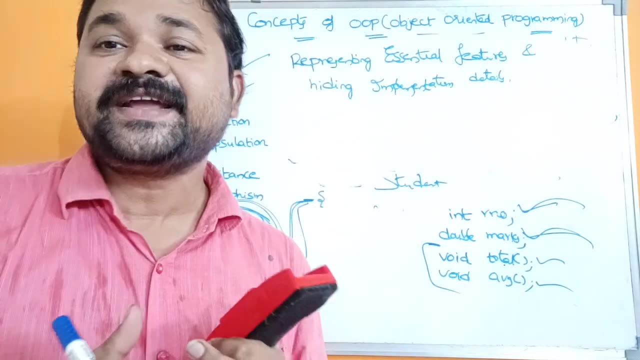 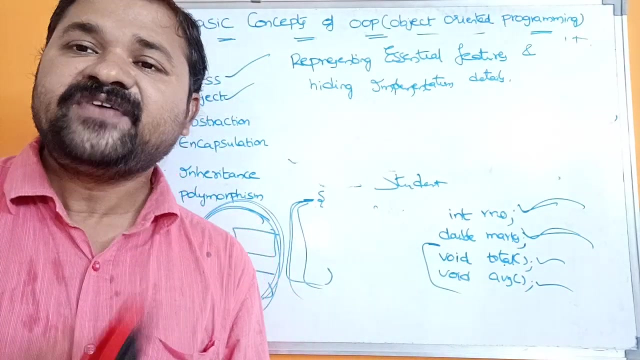 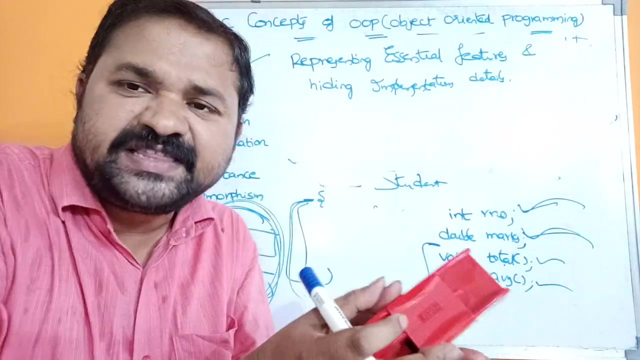 We don't know how the gears are implemented. That is nothing but abstraction. Let's take the example of a fan. We don't know how those internal components of the fan are internally implemented. We don't know how that motor is implemented. If you take the example of a website or a mobile app, we can work with the app as well as we can work with the website. 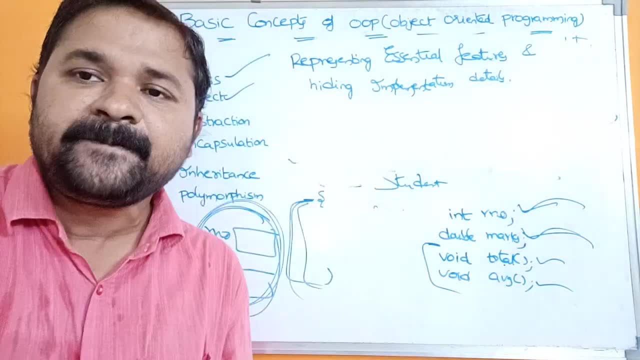 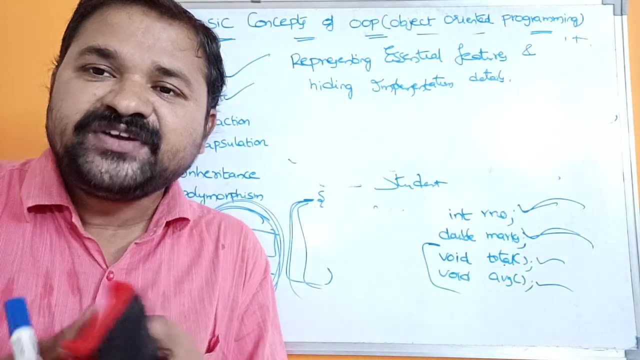 But we don't know how the gears are implemented. website or gap is internally implemented. we don't know which programming language they use it. we don't know which subversive technology they use it. we don't know which database technology they use it. that is nothing but. 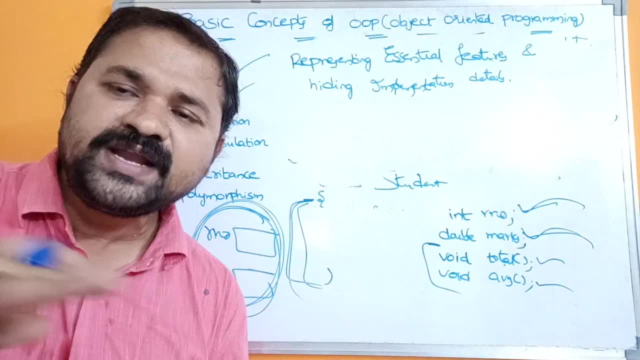 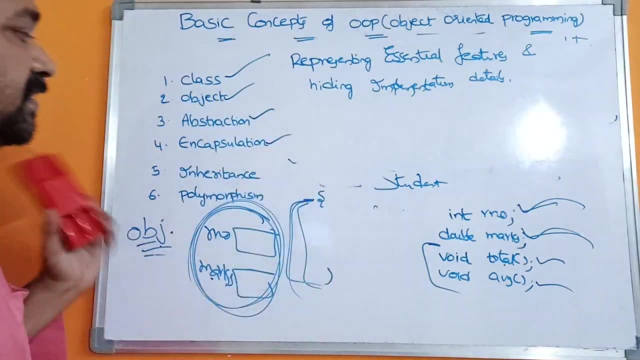 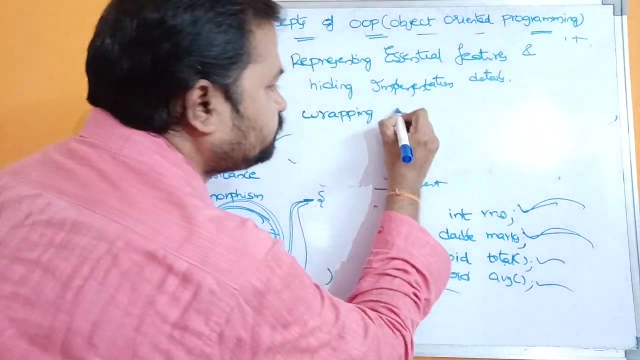 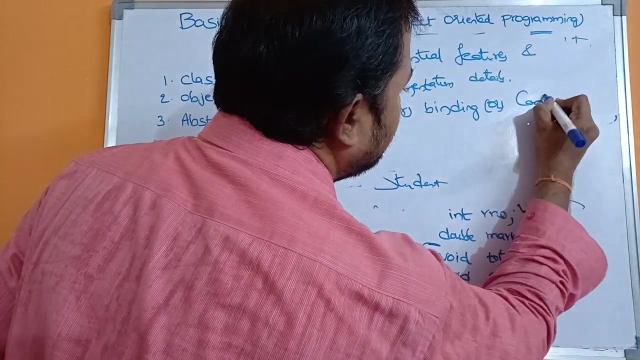 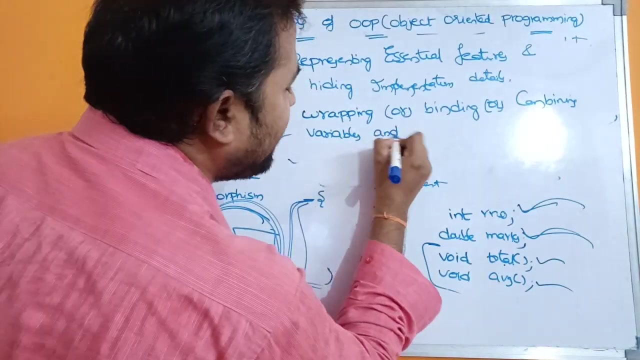 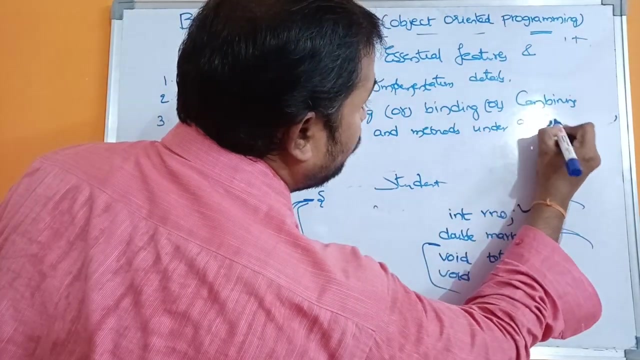 abstraction. abstraction means showing only essential features and hiding the implementation details. now let's see the next one: encapsulation. let's see the definition for an encapsulation. encapsulation means wrapping, or binding, or combining, so combine variables, variables and methods. variables and methods under a single unit, under a single unit called. 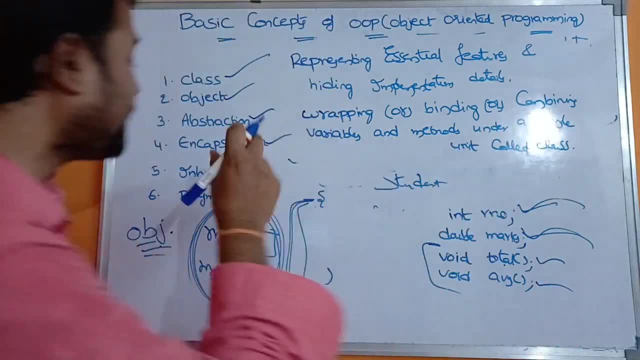 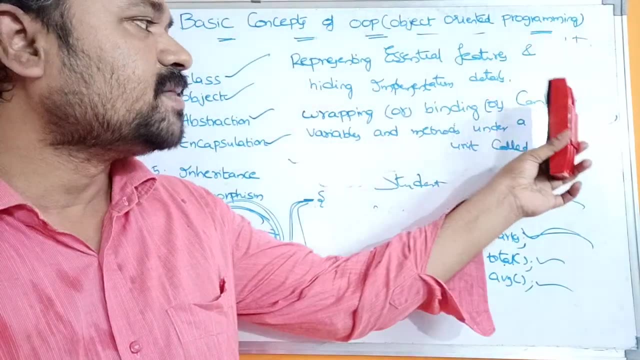 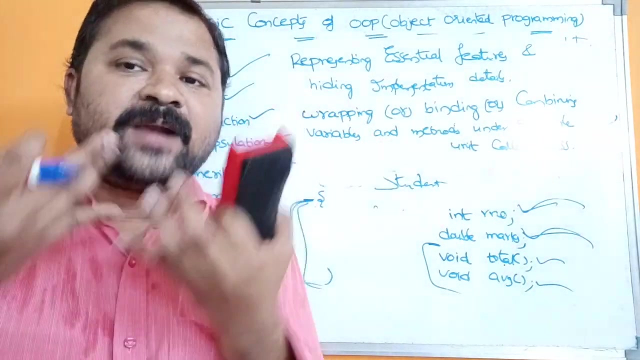 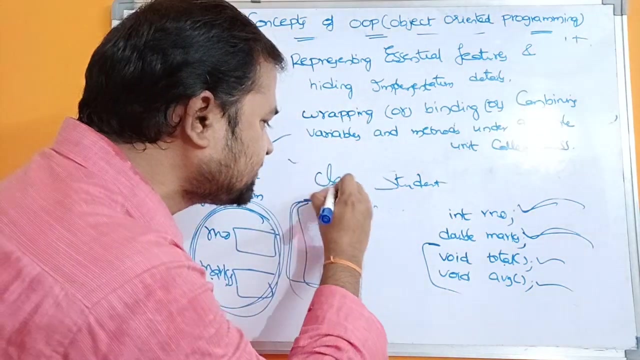 class, class class. so this is the definition for encapsulation. encapsulation is the process of wrapping, or binding or combining variables and methods under a single class. so if we combine, if we place variables and methods in a class, then it is known as encapsulation. so let's see this example. so this is a 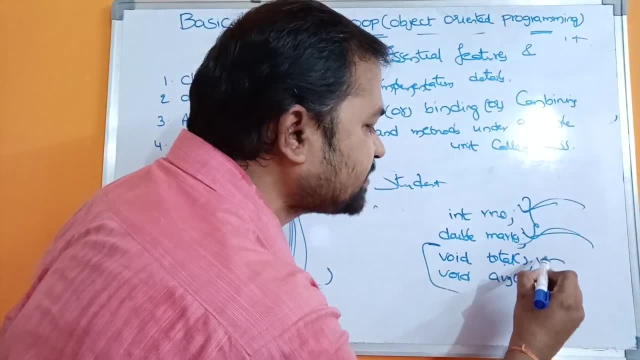 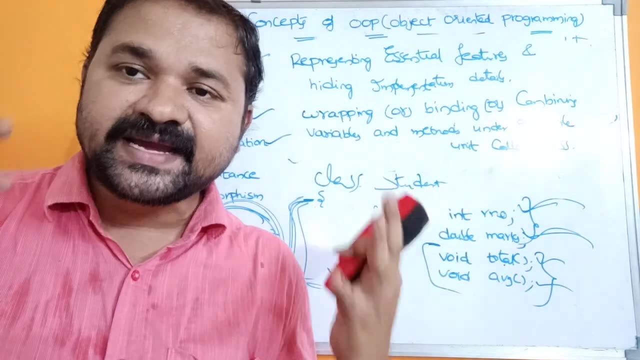 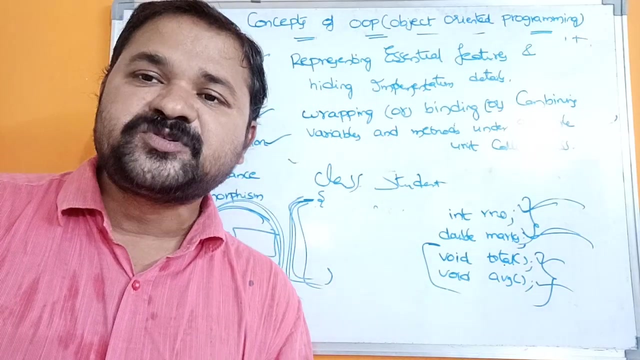 class. so in this class we have variables as well as methods. so this is nothing but encapsulation. so the combining variables and methods under a single unit, under a class, is known as encapsulation. the major advantage of encapsulation is data hiding. so what is the major advantage of? 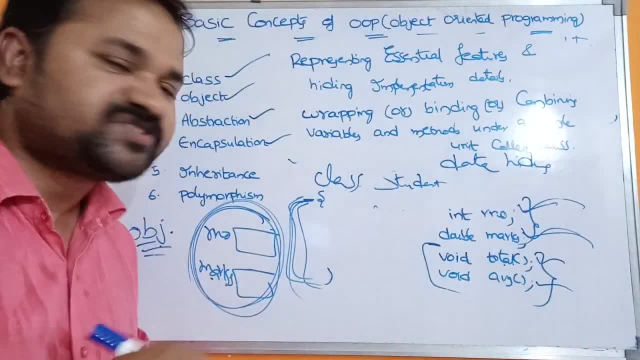 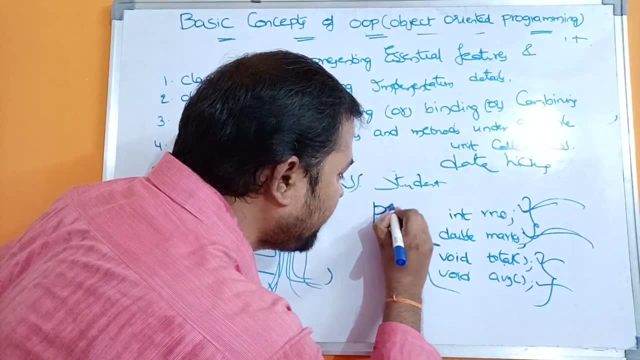 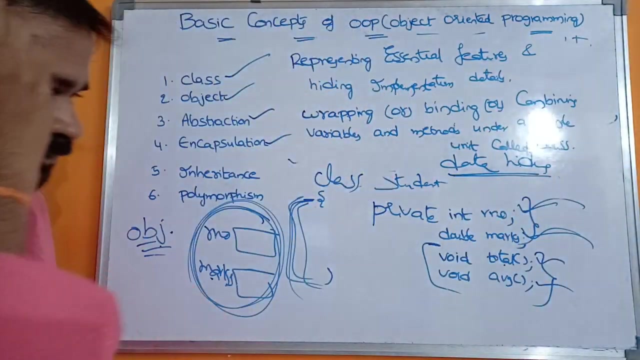 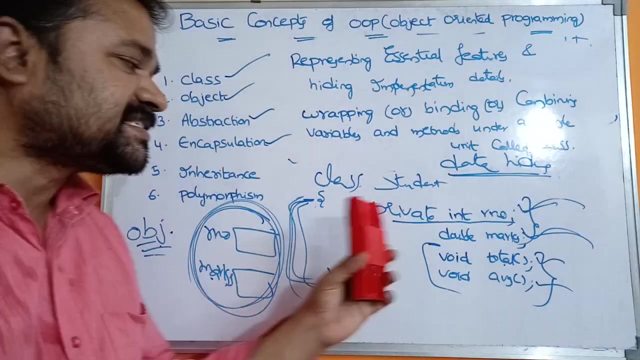 encapsulation data hiding here. we have several access specifiers like private, public, protected and default. we have an access specifier called private, and so private is mainly useful in order to provide data hiding here. let us assume that we have a variable like this: private int rmo. we can access private variable only inside the class. it is not. 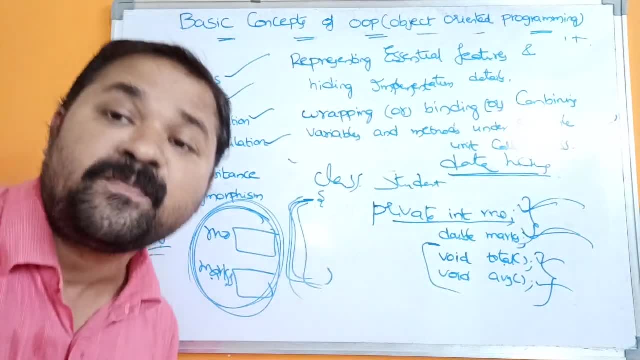 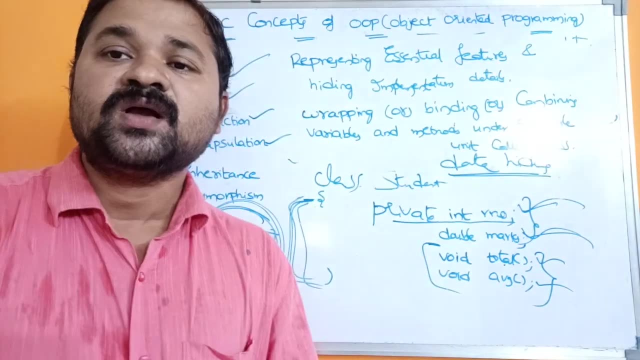 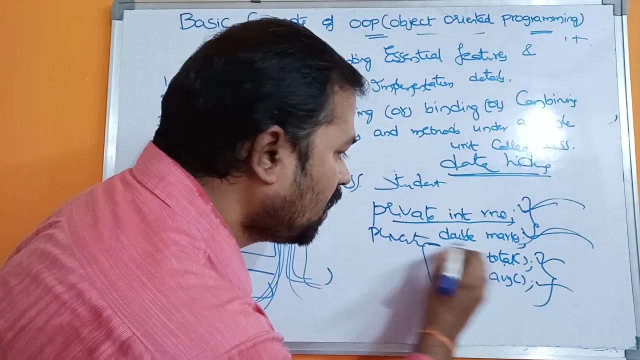 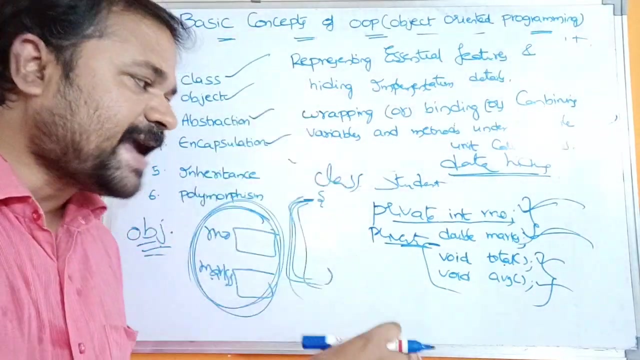 possible to access private variables from outside the class. so that means with the help of the private variable we are providing the data hiding, we are providing security to our data. let us assume that here also mocks is declared as a private variable. so whenever mocks is declared as a private variable, then we can access. 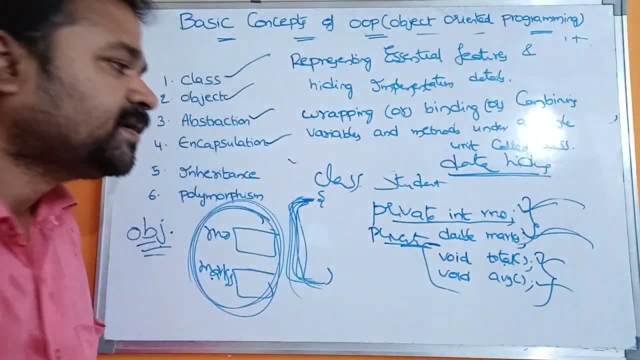 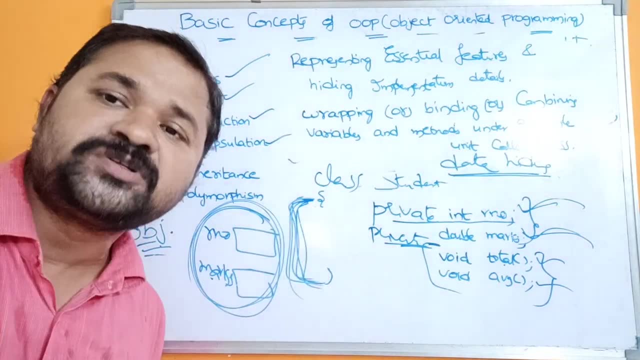 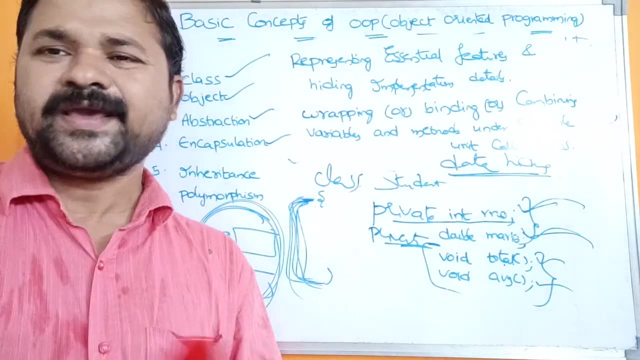 the mocks only from within the class. it is not possible to access mocks from outside the class. if we try to access mocks from outside the class, then the compiler will generates error message. so this is about what is encapsulation. here, mainly, we have two important points. encapsulation is the process of 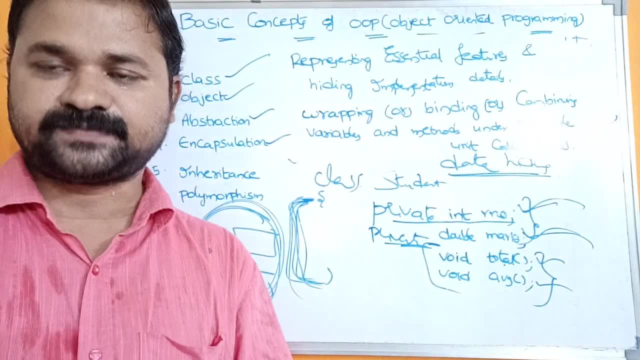 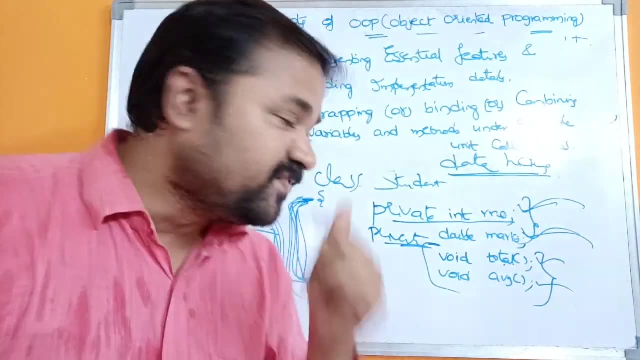 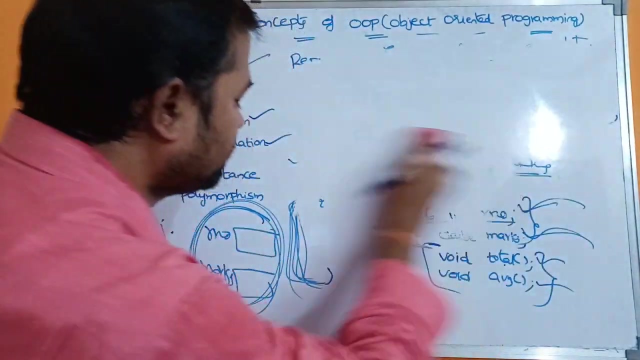 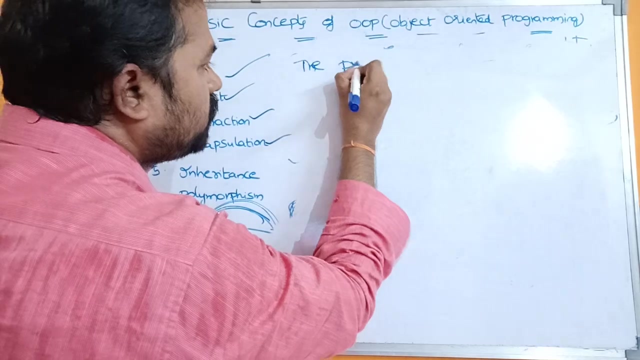 combining variables and methods in a class. the major advantage of encapsulation is data hiding. data hiding is possible with the help of private access specifier. now let's see the next one, that is inheritance. so what is inheritance? inheritance means the process of creating a new class from last class. 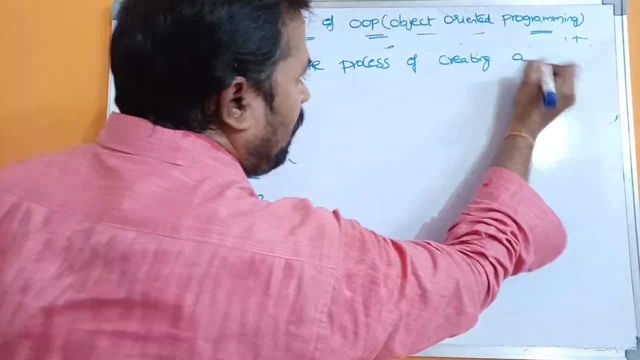 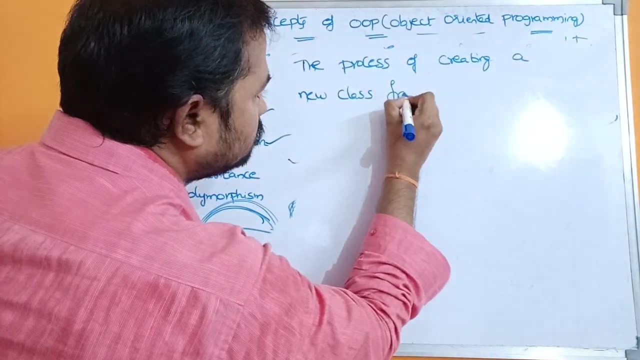 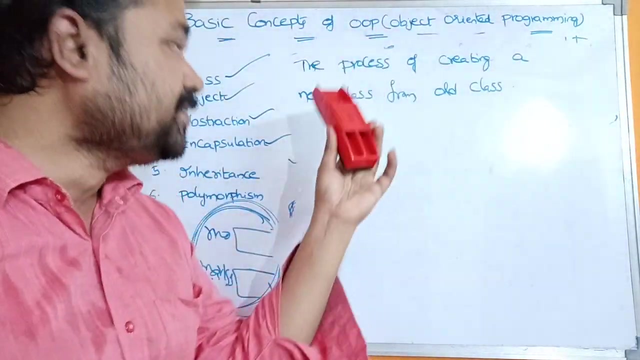 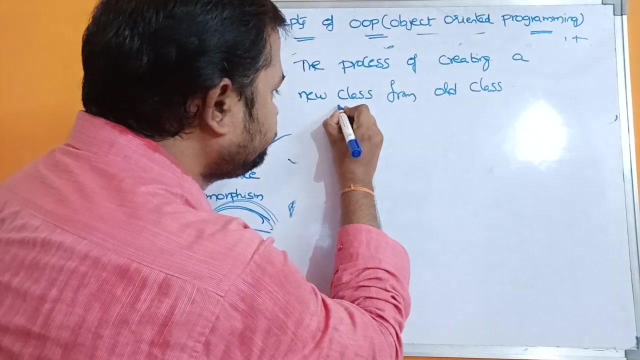 the definition for the inheritance is the process of creating a new class from old class. the process of creating inheritance, the process of creating a new class from old class, is knowledge inheritance. here new class can be called as inheritance a собственn intuitive a어서. 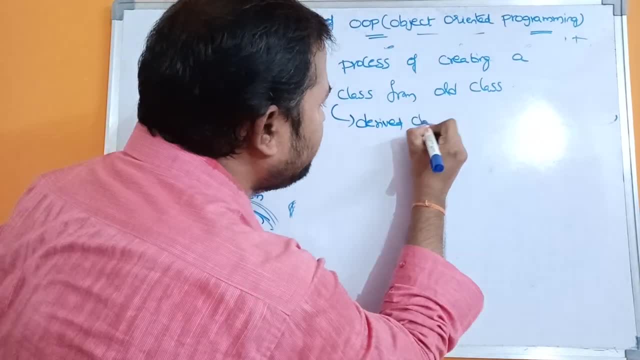 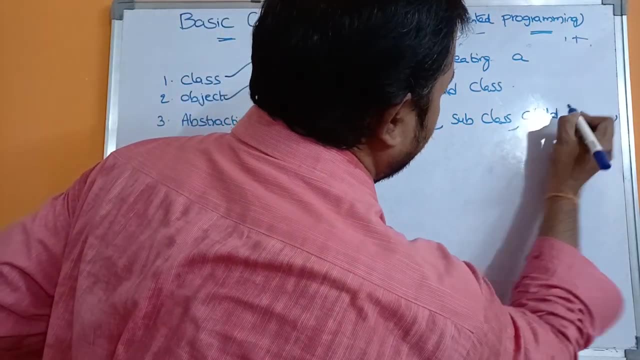 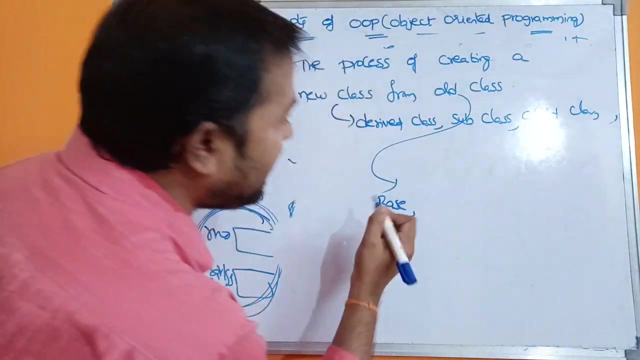 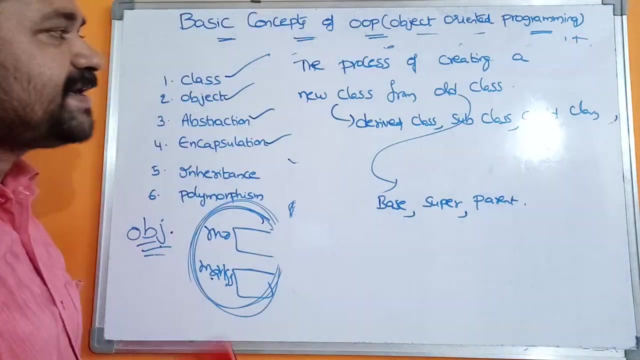 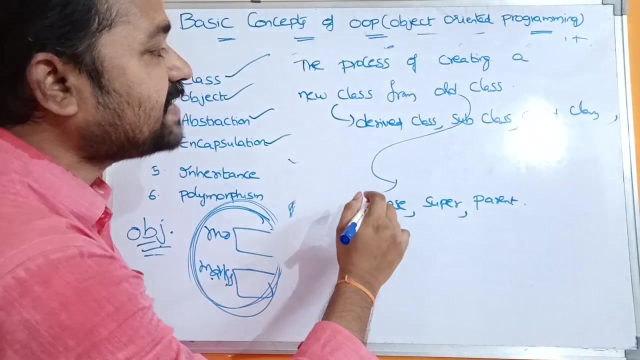 derived class, derived class or subclass or child class. so these three are the various names for the new class. various bold class can be called as base class or super class or parent class. so what is the definition for inheritance creating in new class from the bold class? so we can call the class as: 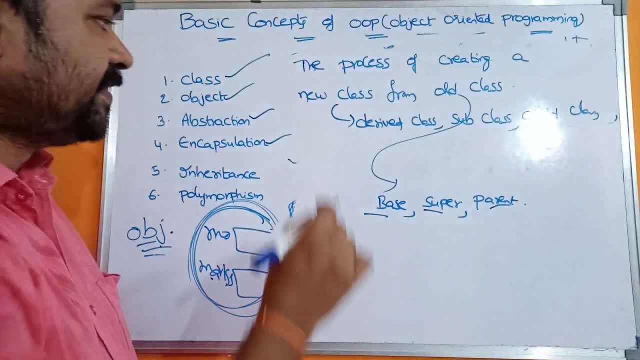 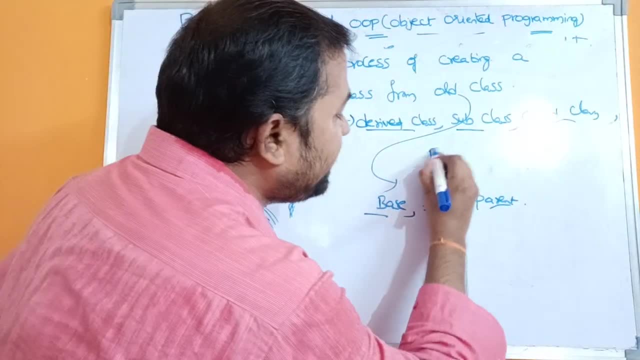 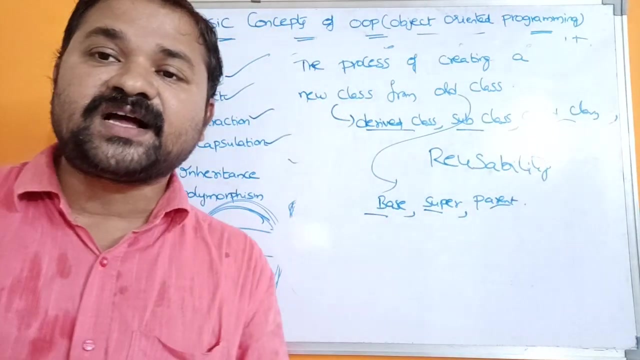 base class, super class, parent class, Varias, we can call new class areas, derived class, subclass and change less. the major evangelism inheritance is reusability. for reusability means reusing the properties of base class, importantly class, so we can use the properties of base class from the derived class. 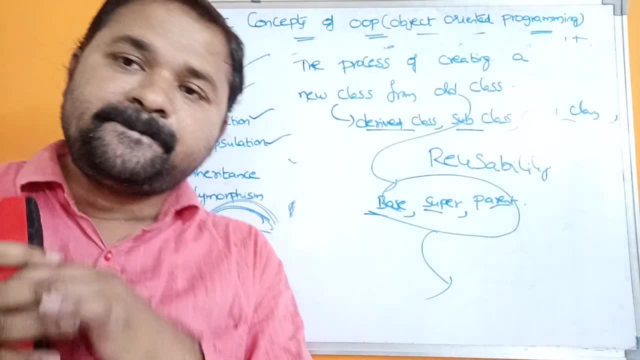 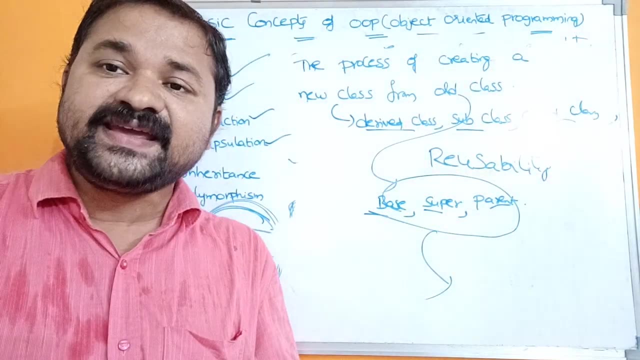 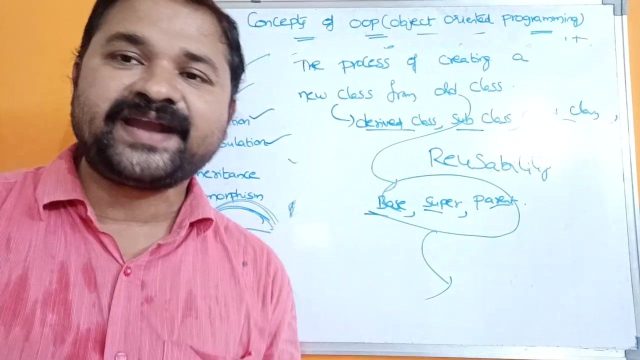 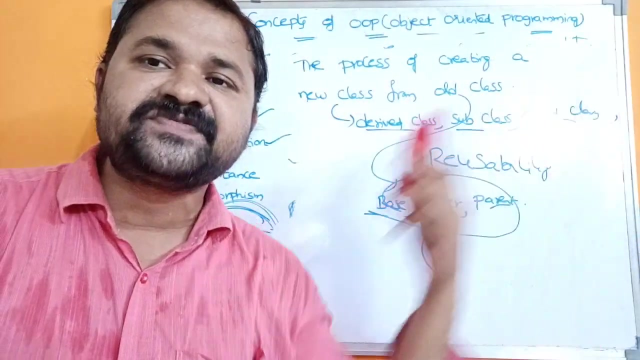 of base class in delivery class. the best example for inheritance is human being. so if you take any human being, then we inherited the features of our parents and our grandparents. we inherited all our facial features and our genetics genes from our parents as well as grandparents, so that 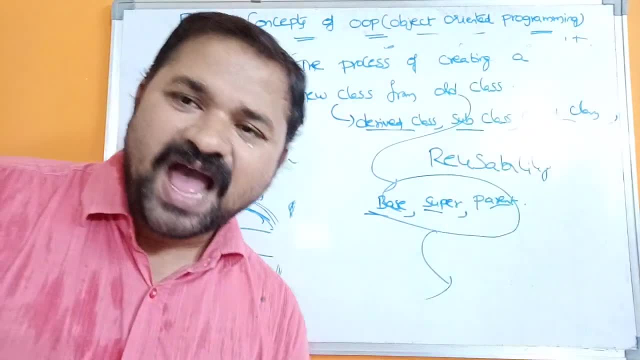 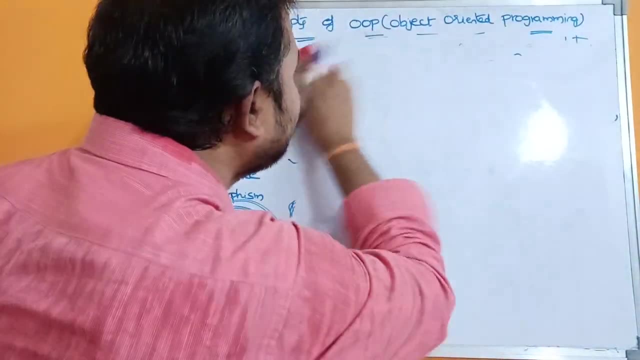 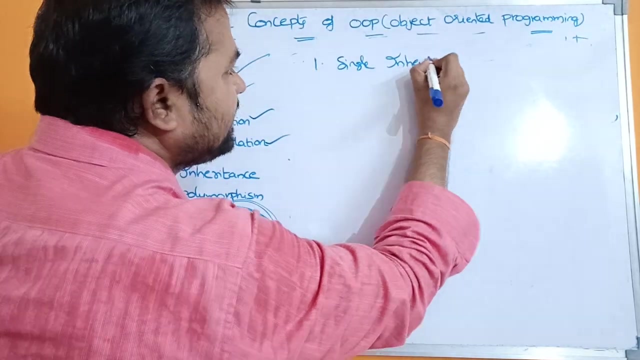 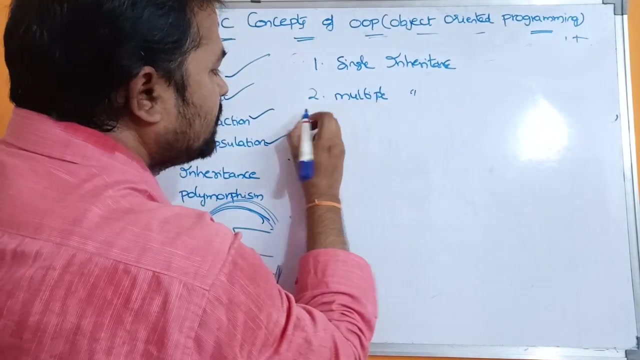 is the best example for inheritance. here we can have several types of inheritance, as larka: single inheritance, multiple inheritance, multi level inheritance, hierarchical inheritance. we can have several techniques. first one is single inheritance. second one is multiple inheritance. third one is multi-level inheritance. fourth one is: 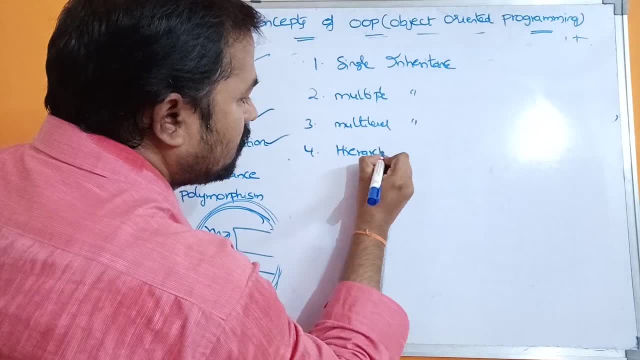 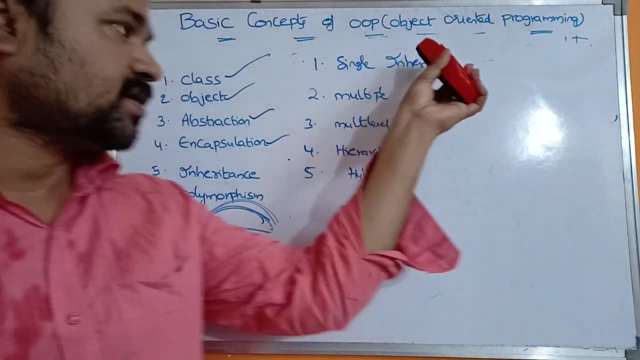 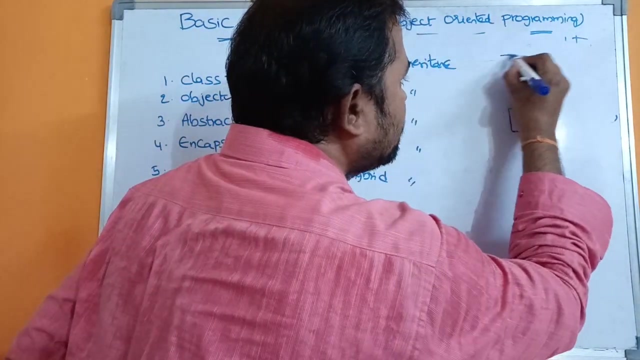 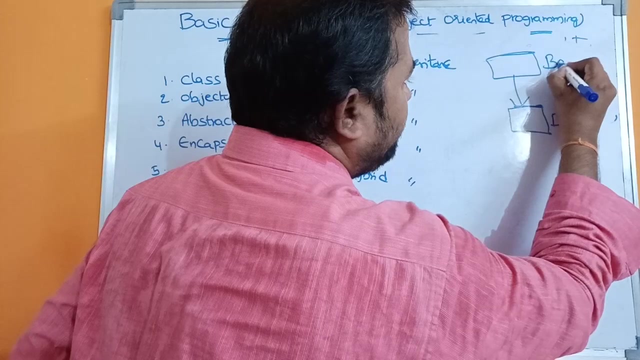 hierarchical inheritance. fifth one is hybrid inheritance. so totally, there are five types of techniques are available. first one: single inheritance. single inheritance means the process of creating a single derived class from a single base class. so this is nothing but our derived class. so this is nothing but our base class: the process of creating a single derived class from a single. 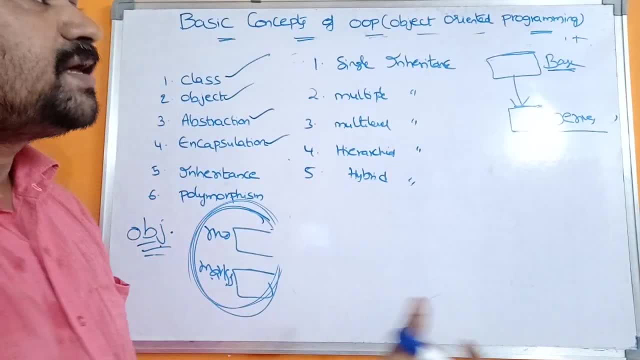 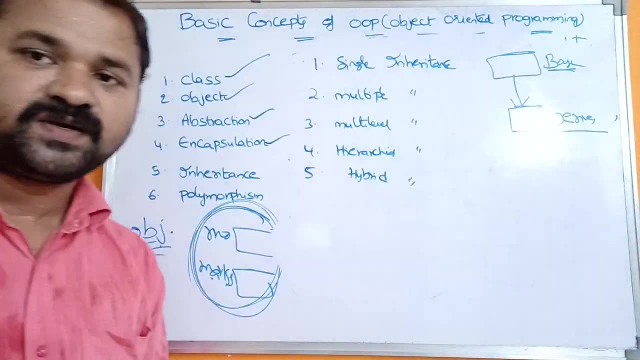 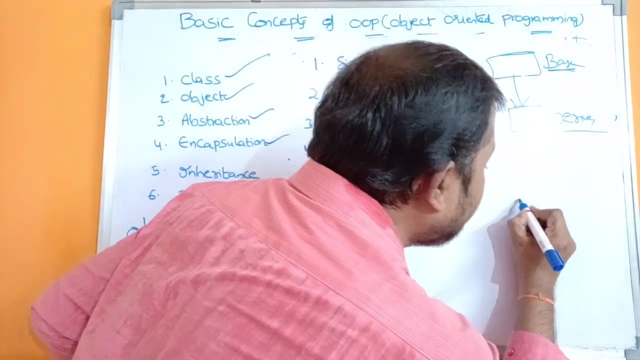 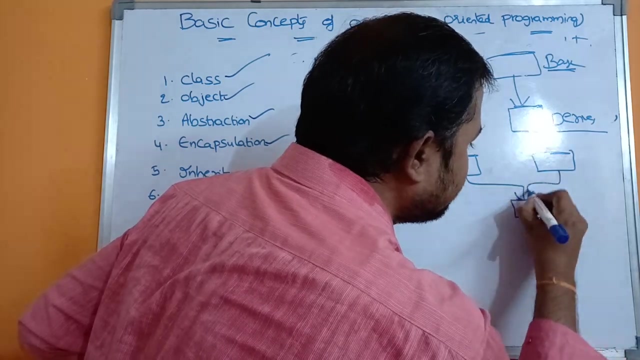 base class is known as single inheritance, so that we can use the properties, the variables and the methods of base class in derived class. we can use all the variables of based clase derivative class. let's the second one: multiple inheritance. multiple inheritance means the process of creating a derivative class from multiple base classes. so this is nothing. 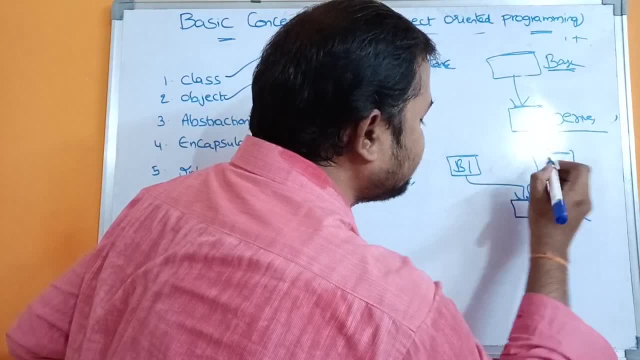 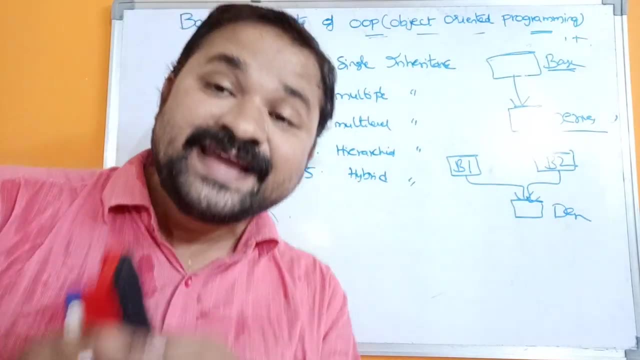 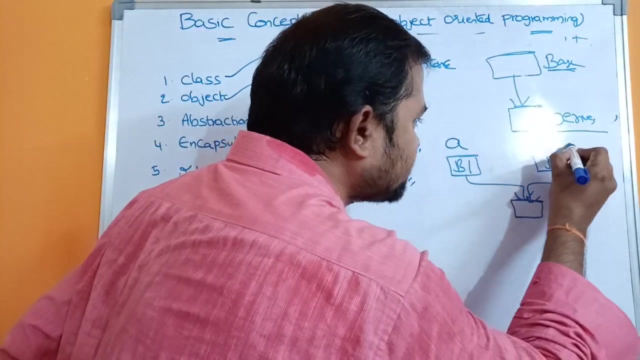 but our beginning class where, yes, this is nothing but our base class mode. this is but our base class 2, but java language doesn't support multiple inheritance. why java language doesn't support multiple inheritance? let us assume that base class 1 and base class 2 contains a. 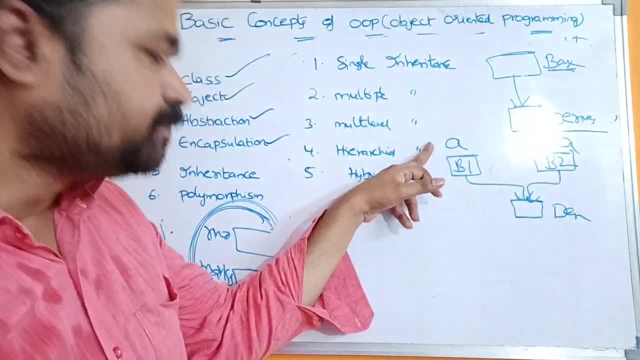 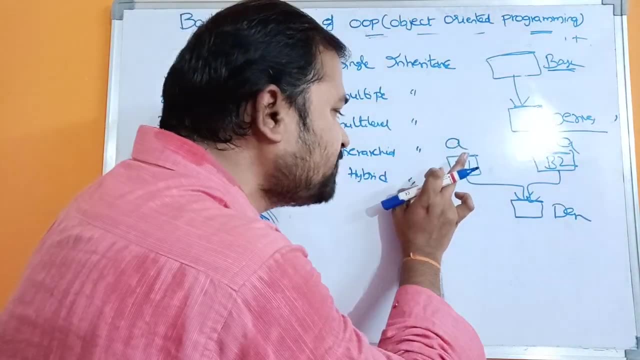 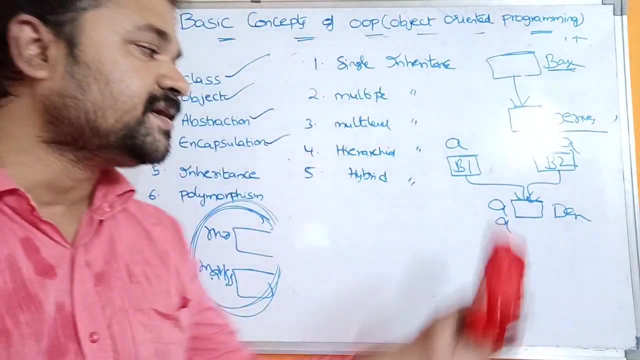 common member variable. here we have a variable called a which is present in base class 1 and base class 2. so if we create a derived class by extending from, by inheriting from base class 1 and base class 2, then multiple copies of a are available in derived class. so if we try to access 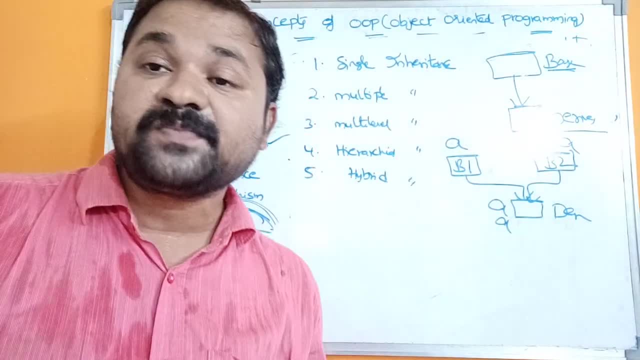 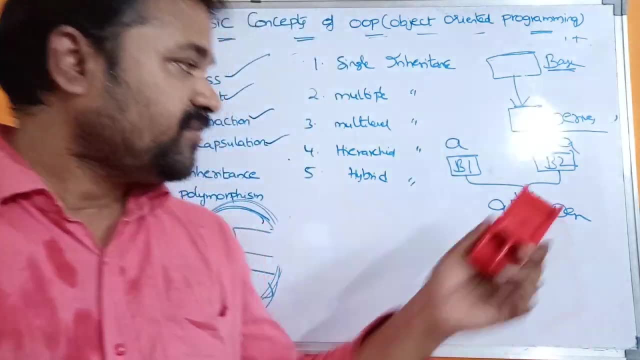 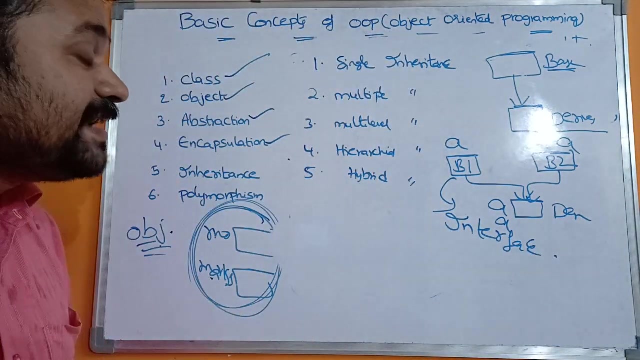 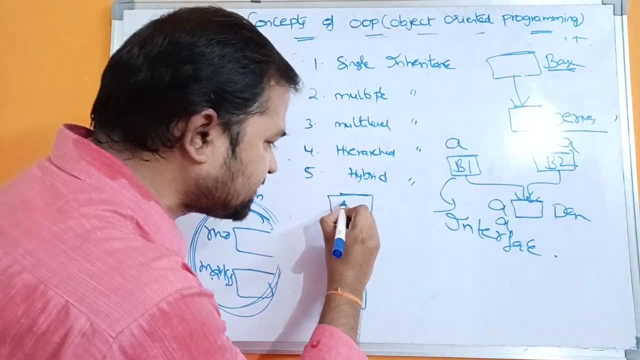 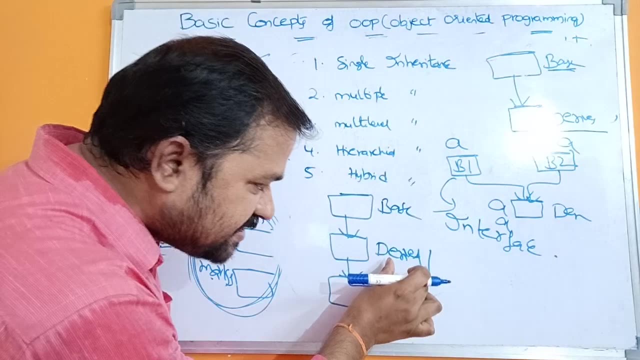 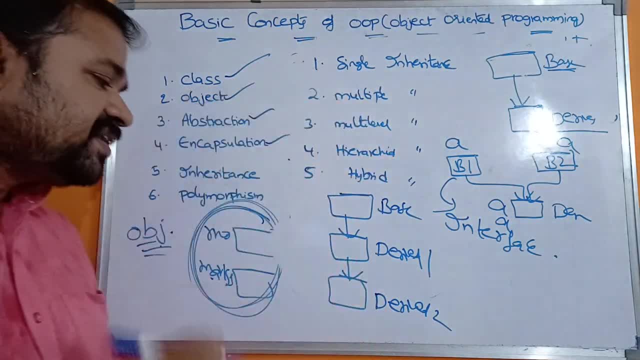 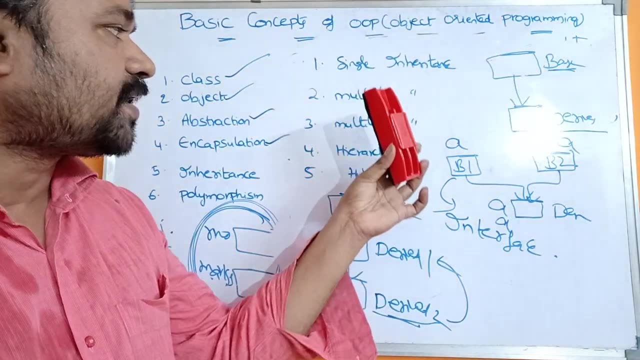 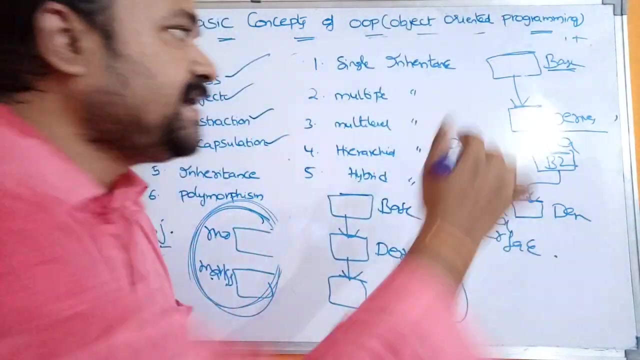 class. so multi-level inheritance means the process of creating a class from the derived class. if you take single inheritance or multiple, or hierarchical, always we have to create a derived class from the base class. here this is the base class, these two are the base classes. but here what we are doing, we are creating. 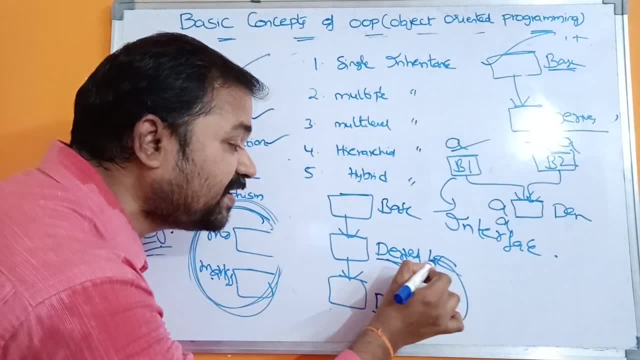 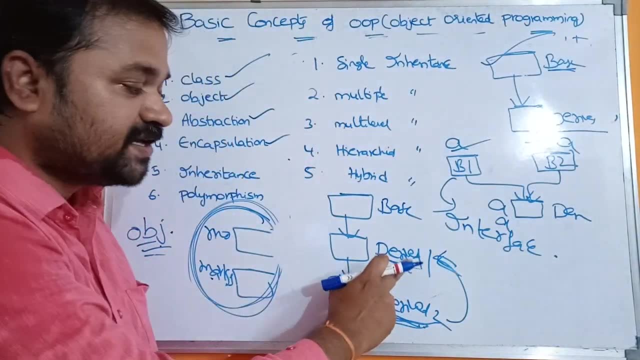 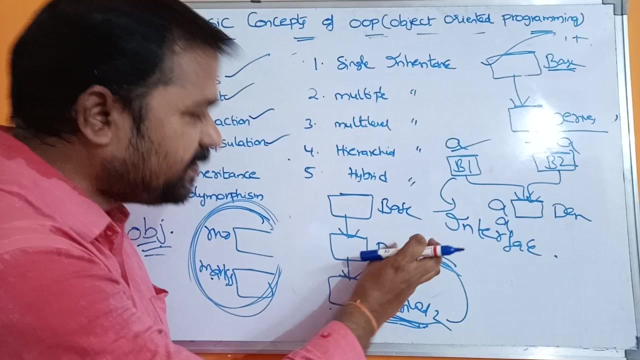 derived two class from derived one. but derived one is what derived class? so first, this is the base class, so from this base class we have created derived one class. next, this derived one class acts as a base class for derived two. so we have created derived two class from derived one. next, 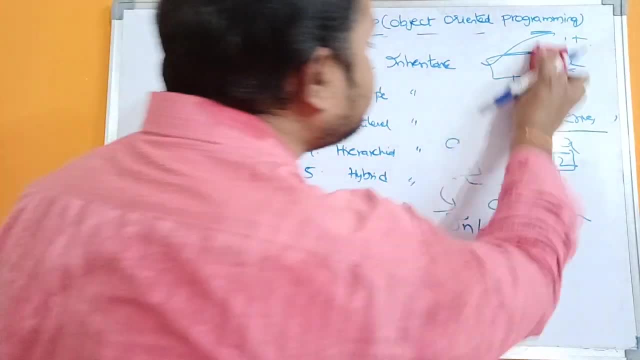 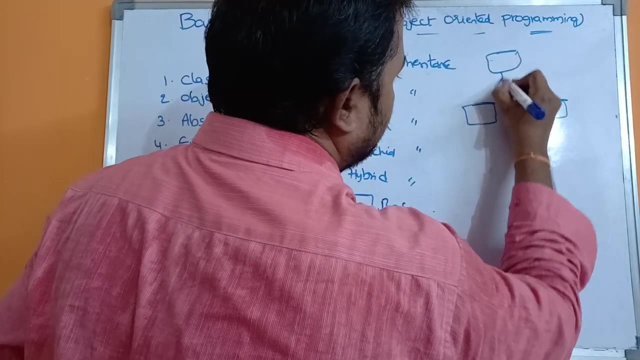 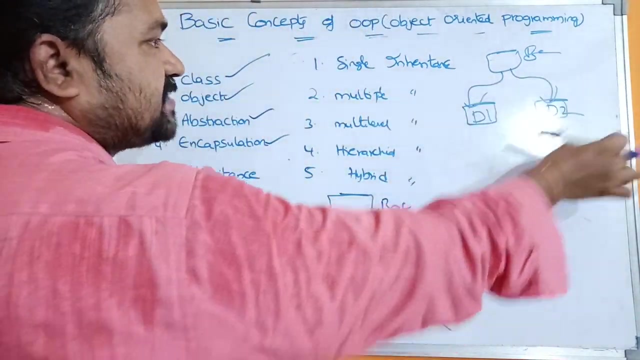 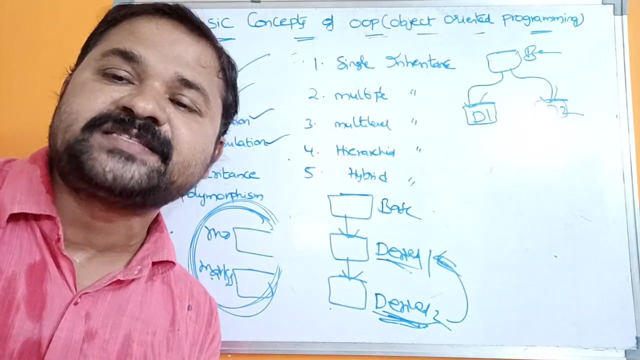 one is hierarchical inheritance. so hierarchical means the process of creating several classes from the single base class. so this is nothing but our base class. this is derived one class, this is derived two class. so creating several classes from the single base class is nothing but hierarchical. next one is hybrid inheritance. hybrid inheritance means it is a combination of more than one type of 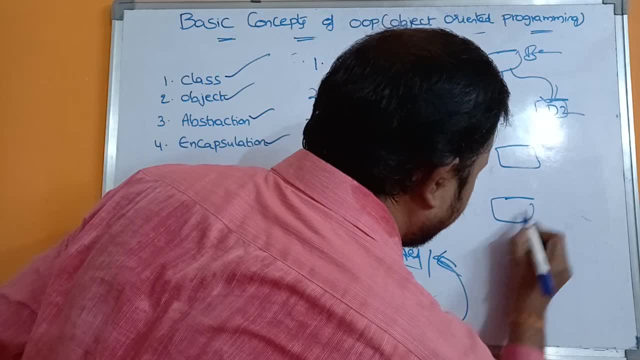 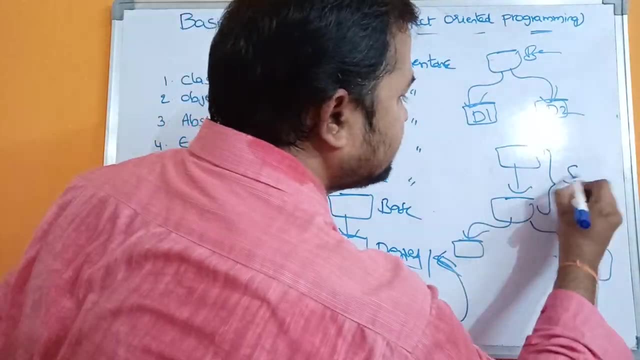 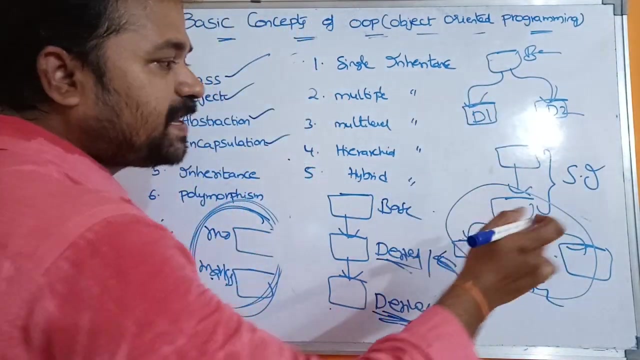 inheritance. so let me have a diagram like this: okay, so this is nothing but hybrid inheritance. so if you take this one, so this is nothing but what single inheritance, whereas what is this one? this one is nothing but hierarchical inheritance, so this diagram involves single inheritance as well. 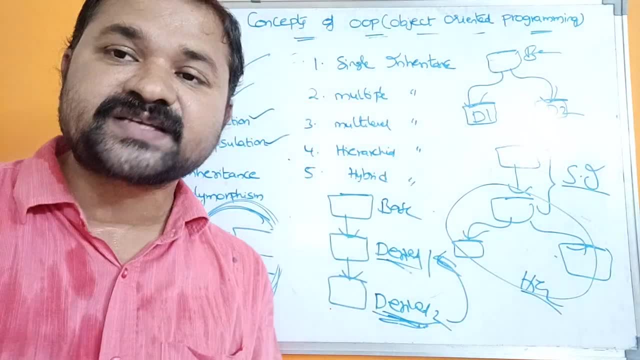 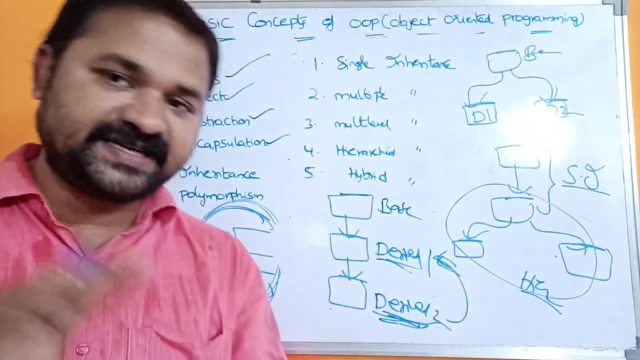 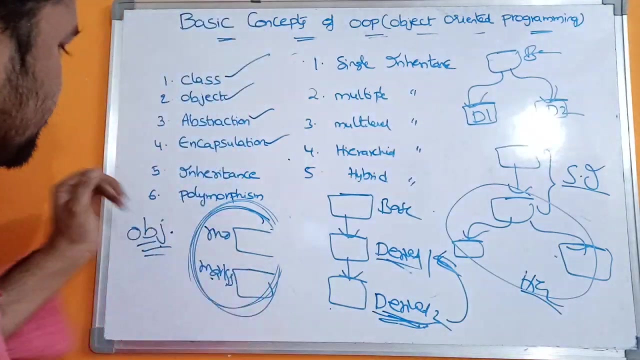 as hierarchical inheritance, so that's why this is known as hybrid inheritance. so hybrid inheritance is a combination of more than one type of inheritance. so this is a combination of more than one type of inheritance. but if it contains multiple inheritance, then it is not possible to implement the diagram. so this is about inheritance. now let's let's see the last basic concept of 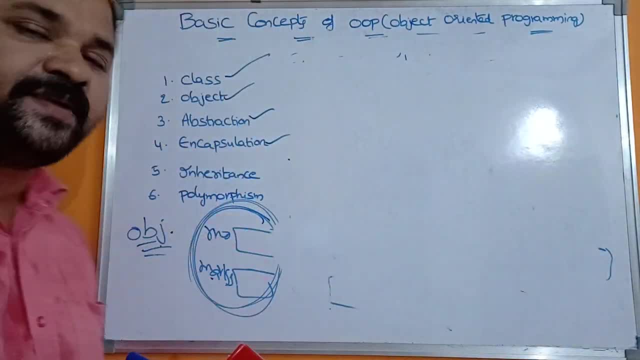 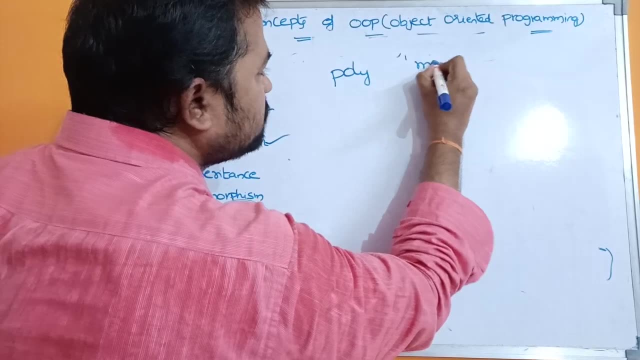 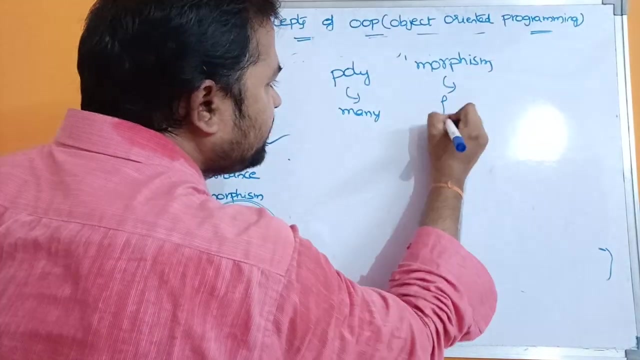 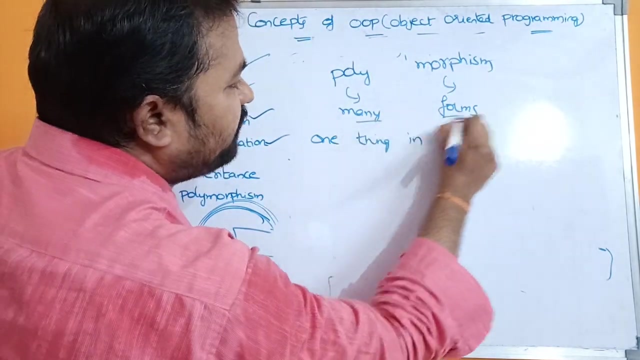 object-oriented programming, that is polymorphism. polymorphism is derived from two Greek words: poly and morphism, so these two are Greek words. poly means many various. morphism means poly and morphism, so these two are Greek words. poly means many various. morphism means force, so representing one thing in many forms. representing one thing in many forms is called